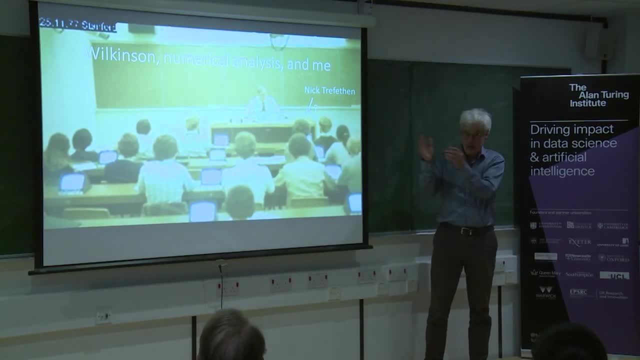 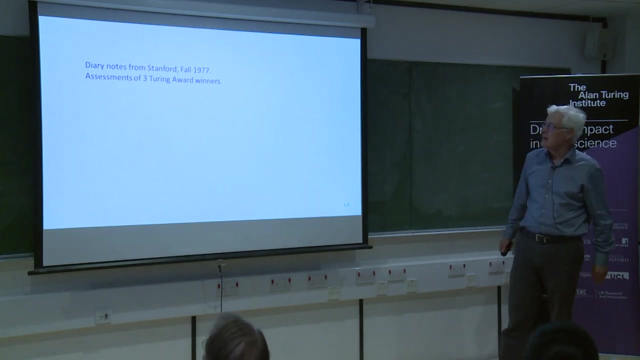 And in my notes I even mentioned one time this was being filmed by the cameraman Once he had gone over so long that the cameraman moved the camera and pointed at the clock. So I want to begin with some notes from my diaries in those days. 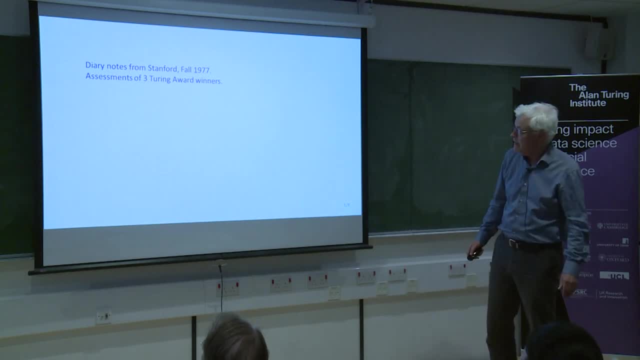 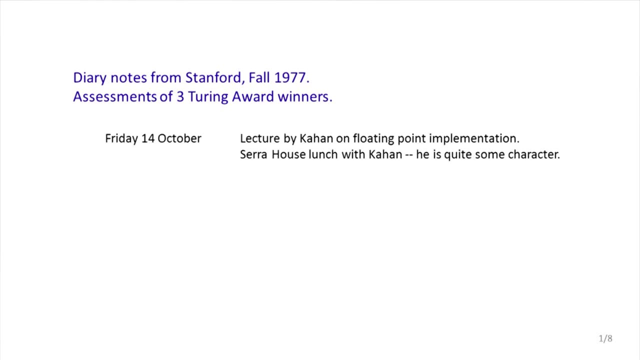 And just I'm going to mention three things I scribbled down about people who had already won or were destined to win Or were destined to win, the Turing Award. So this is the 14th of October, 77. Lecture by Cahan on Floating Point Implementation. 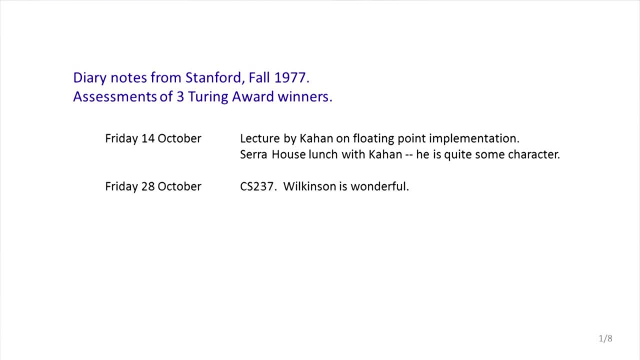 He is quite some character. 28 October Wilkinson is wonderful, And this was the course. So this is that fall of 1977.. And then John McCarthy, this great genius. Oh God, he was an awful. He called it Uncle John's Mystery Hour. 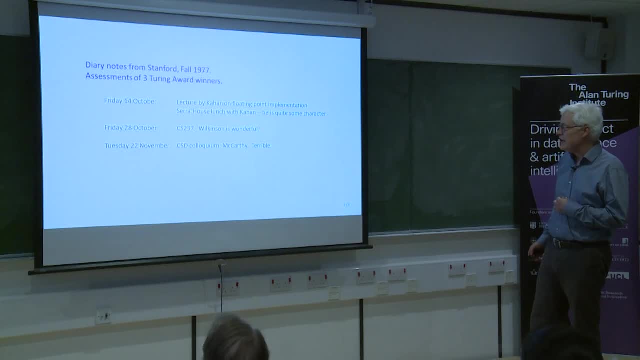 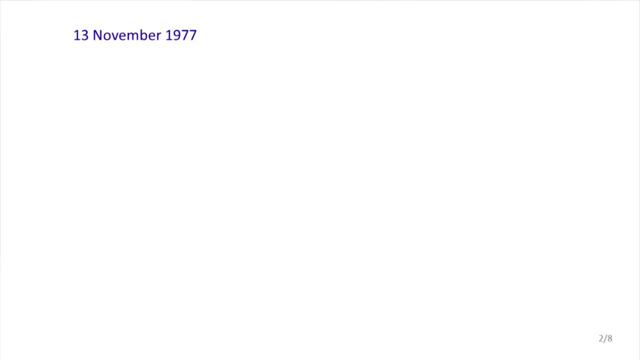 Okay, Right, So in this talk- Oh sorry, A little more- I wanted to show you of diary stuff, So this is actually scanned in from. I was a mad typist, So at last Thursday's lunch Wilkinson, Householder and Golub were all very present. 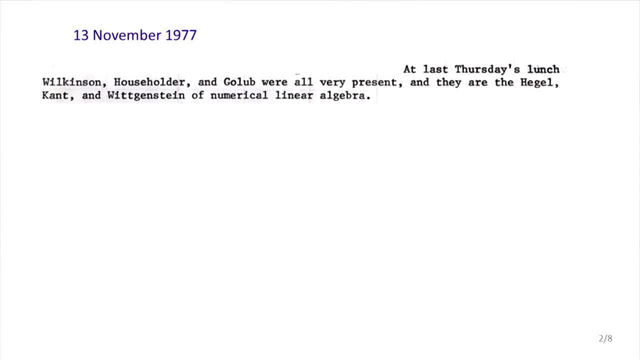 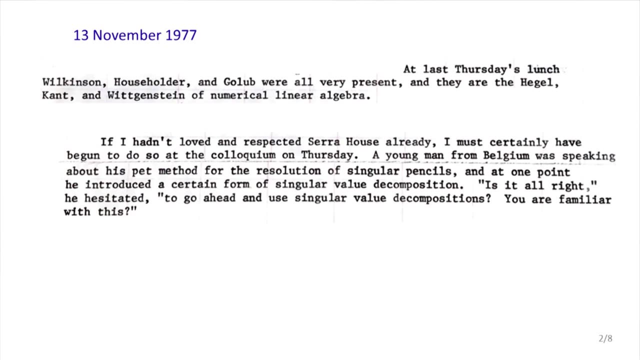 And they are the Hegel, Kant and Wittgenstein of numerical linear algebra. And this is later in that same diary entry. If I hadn't loved and respected Serrahaus, which is where we all were already, I must certainly have begun to do so. 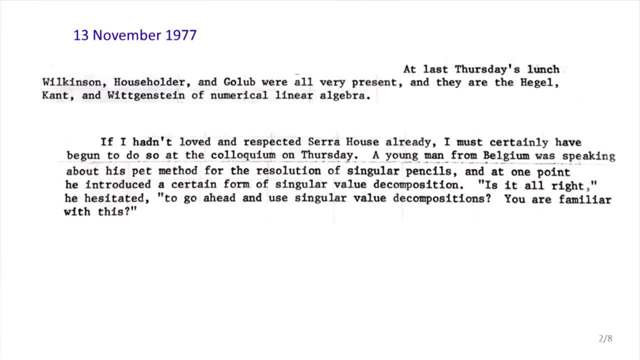 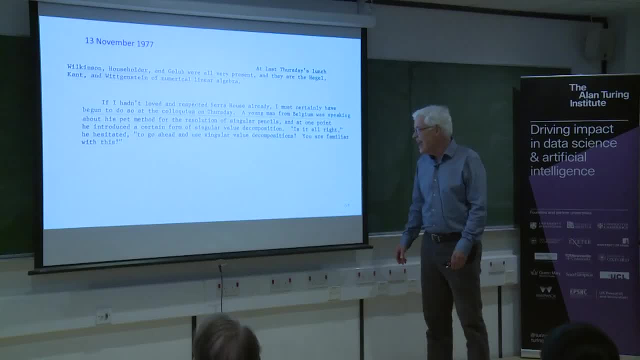 at the colloquium on Thursday, A young man from Belgium was speaking about his pet method for the resolution of singular pencils- Can anyone guess who that might be? And at one point he introduced a certain form of singular value: decomposition. Is it all right? he hesitated. 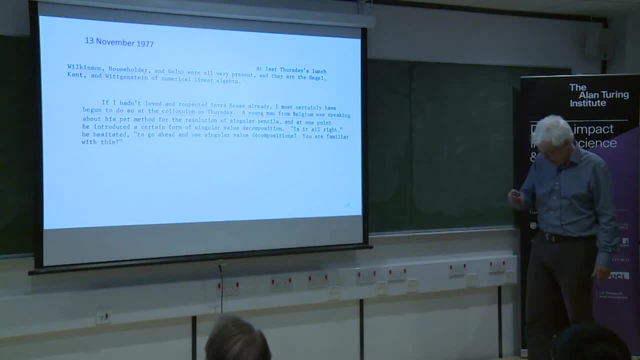 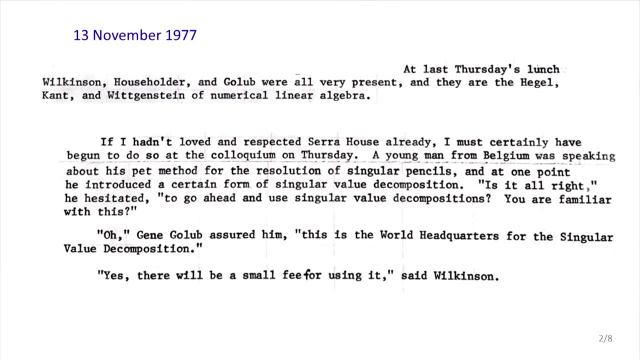 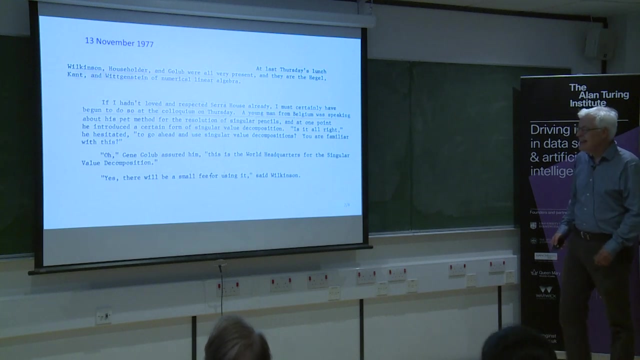 to go ahead and use singular value decompositions. You are familiar with this. Oh, Gene Golub assured him. this is the world headquarters for the singular value decomposition. Yes, there will be a small fee for using it, said Wilkinson. And that was so typical. 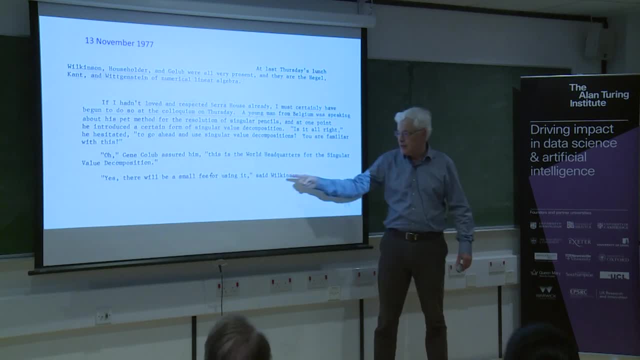 I'm two months into my graduate career, but you can see I love this guy, right? I wasn't writing this stuff in order to impress you 40 years later. I really loved the man, Okay, so in my talk I wanted to mention: 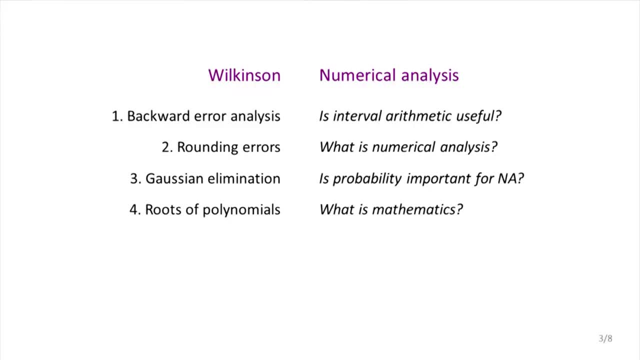 four topics, each one very briefly, Four things of passionate importance to Jim And in each case I want to use that as a springboard for a question that has interested me and that might interest you, related to numerical analysis, Because of course, Jim was the great numerical analyst. 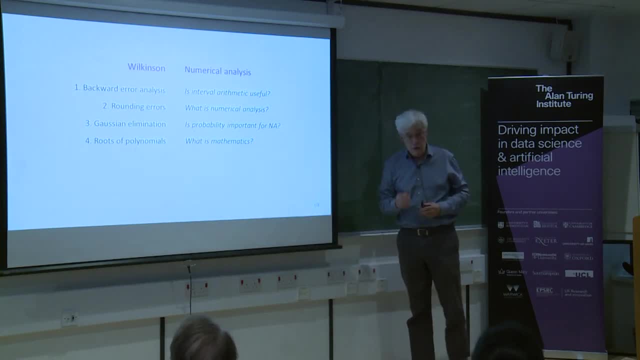 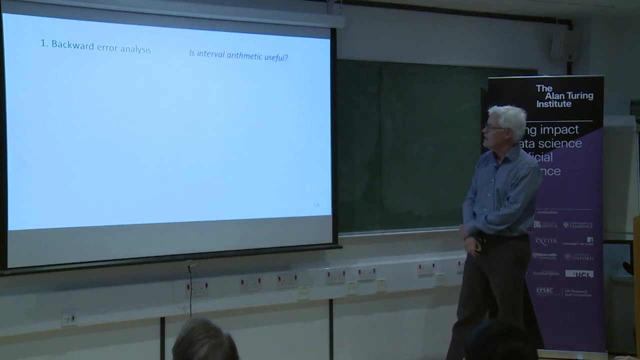 of his era. one of them: He was not only interested in linear algebra, but he epitomized numerical computation. So the four topics: Backward error analysis, rounding errors, Gaussian elimination and roots of polynomials. So let's begin with backward error analysis. 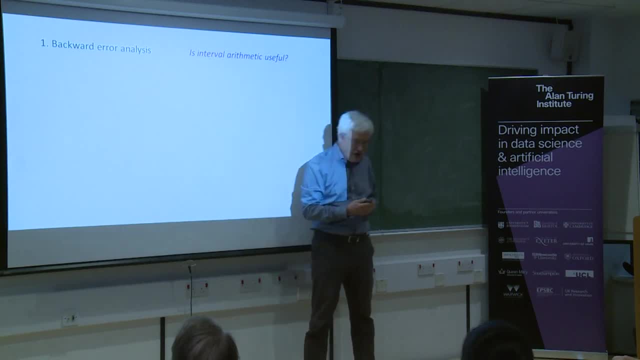 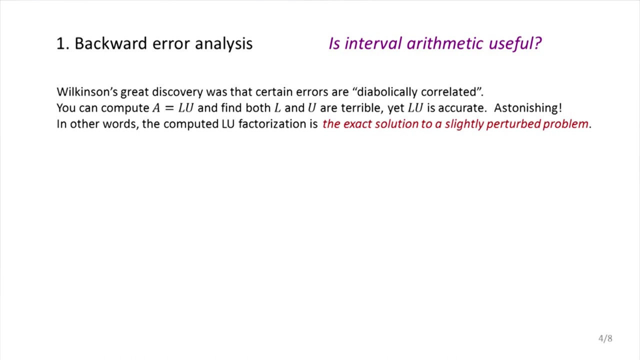 And the question that I want to connect that to is the question of whether interval arithmetic is useful. Does anyone here do interval arithmetic? Uh-huh? Well, that already says something about a separation between two fields, doesn't it? So, as several people have mentioned, 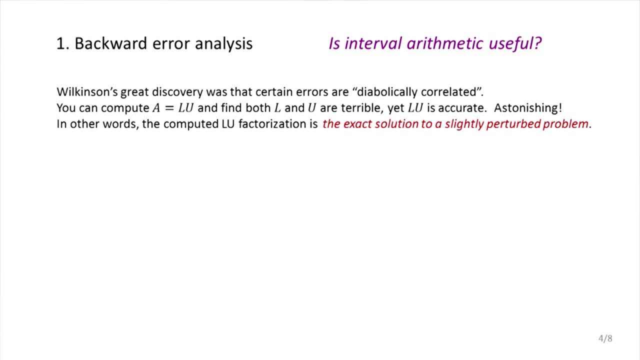 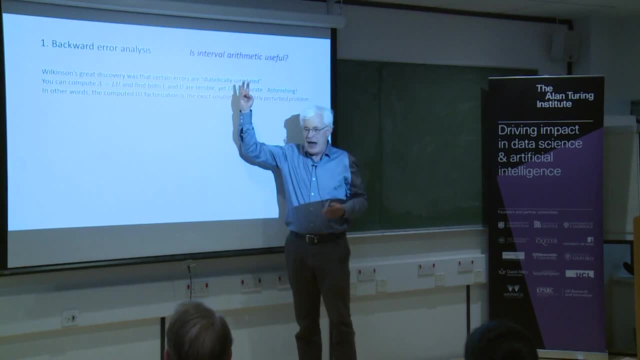 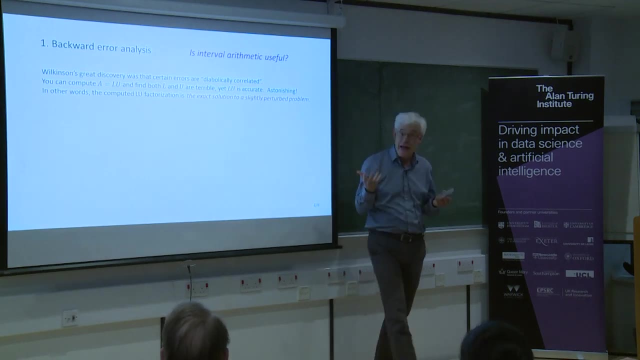 and Margaret. your talk said this so nicely, Wilkinson, really the pivotal exciting discovery of his career was this diabolical correlation of errors between things, And I always think of it in terms of AX equals B, but Margaret showed us that maybe the eigenvalue problem. 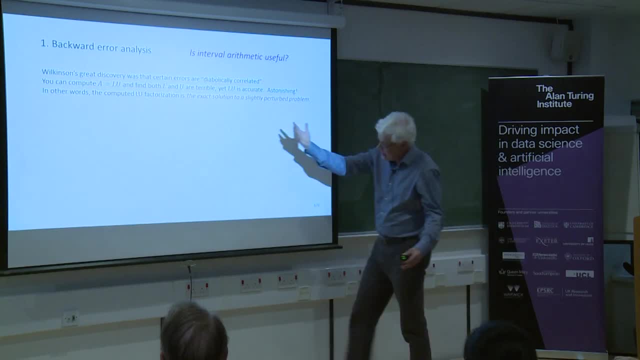 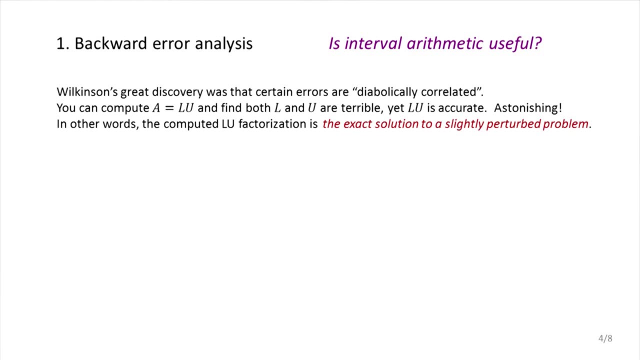 was even more fundamental. So in AX equals B terms, you can compute A equals LU. Well, it's probably pivoted, but I'm ignoring that And you'll find that L is awful and U is awful, And yet L times U is fine. 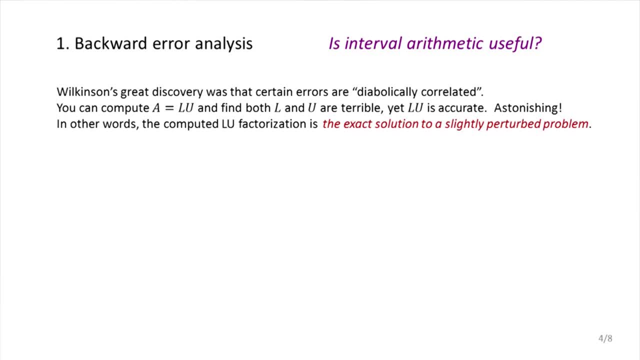 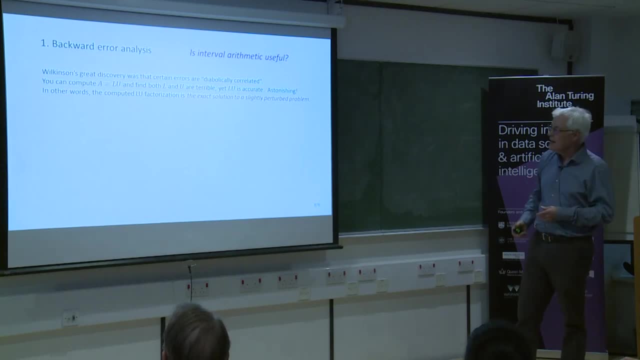 And this is totally a Wilkinson phrase. He said: L has big errors and U has big errors, but the errors are diabolically correlated to have this amazing effect that the product LU is fine. So you get a computed LU factorization. 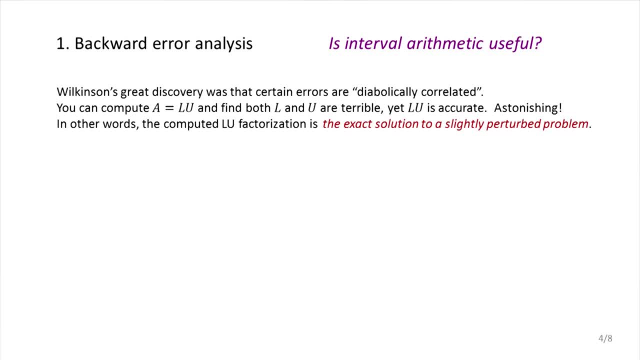 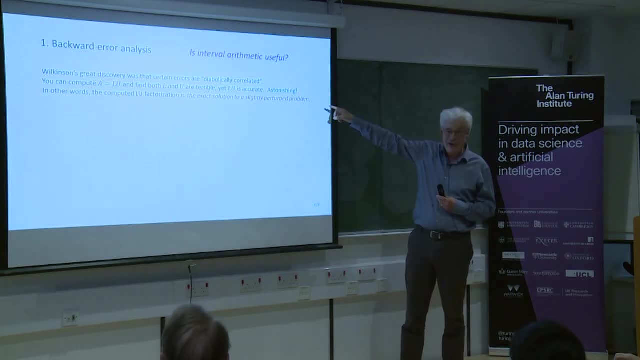 which is the exact solution to a slightly perturbed problem, And that was. I'm sorry I couldn't find you, Margaret. I didn't realize till your talk that great quote where he says backward error analysis was good marketing, but now he would emphasize it less. 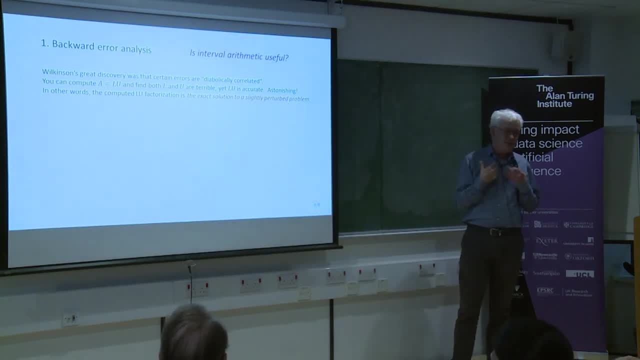 That's really interesting, But there's no doubt this was the pivotal discovery of his career And he found that it worked for eigenvalues and for AX equals B and for roots of polynomials. It was an amazing thing for him to find that. 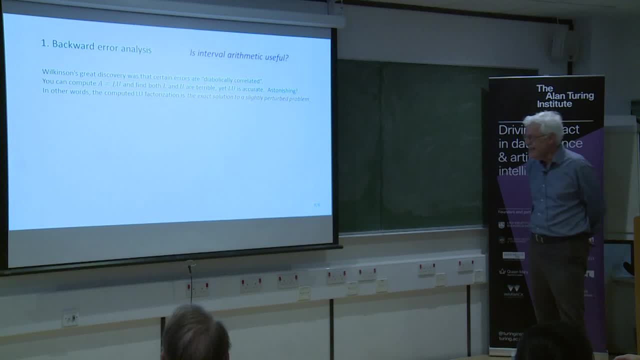 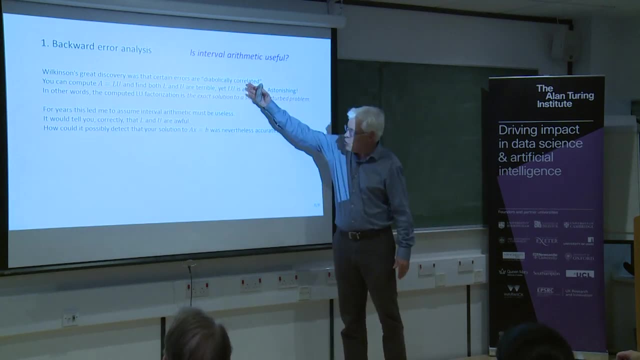 Yeah, it took them generations- Good point. So I absorbed this deeply because this was my first experience as a graduate student. You know, Jim really affected me And one of the conclusions that it led me to was an assumption: that interval arithmetic. 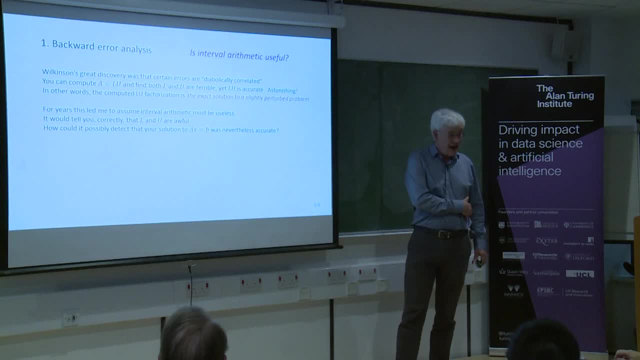 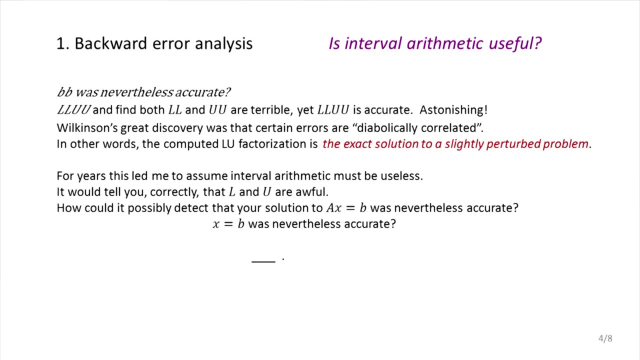 although very pretty, must be useless in practice. I don't actually know what Jim thought of interval arithmetic, So let me spell out the idea here. If you do interval arithmetic, it's going to rigorously track how big your errors are. 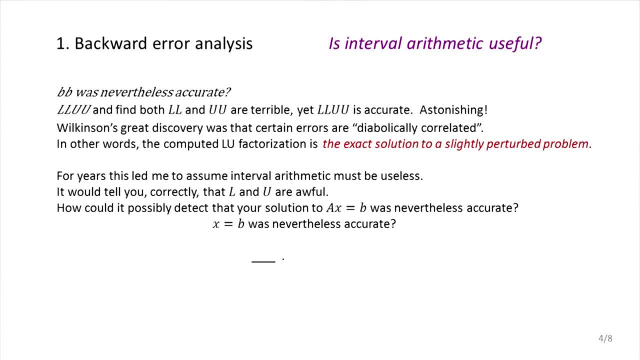 So, of course, it'll tell you that L is awful, and it will tell you that U is awful, and it will be right. So, in that context, how are you ever going to know that in the end, you've got the right answer? 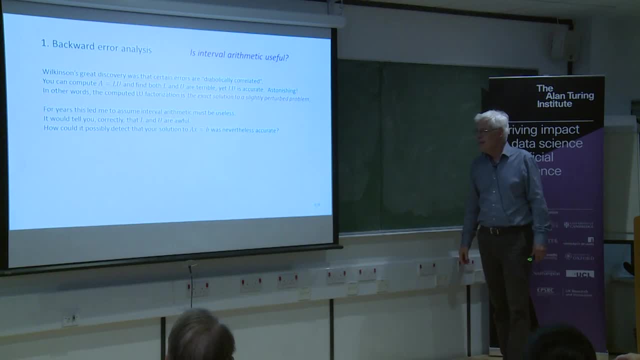 So I think I spent about 20 years believing that interval arithmetic was a beautiful, useless idea. I think John knew better all that time. Various people knew better, Many people knew better. I was missing the point, And maybe some of you, if you think about it. 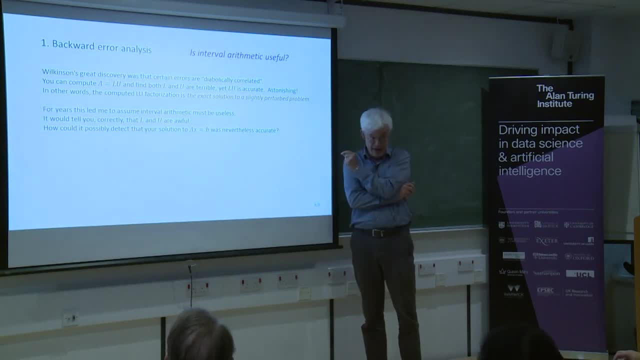 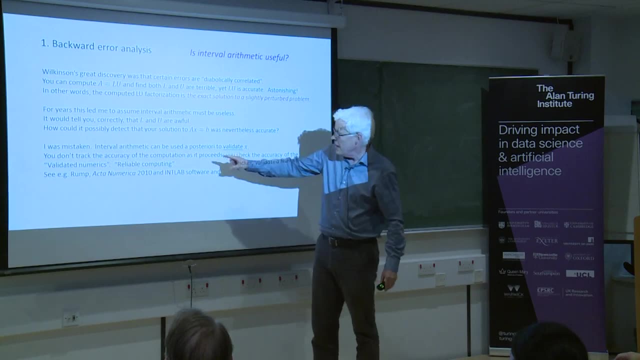 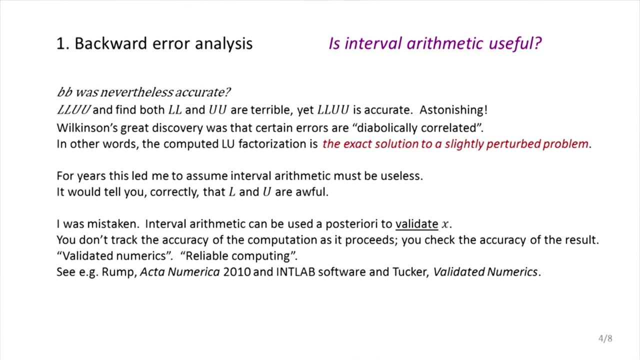 I'm sure many of you know what the flaw in this reasoning is, and maybe some of you don't. So the flaw is that actually, interval arithmetic can also be used in an a posteriori way. So you compute your x, You don't track anything. 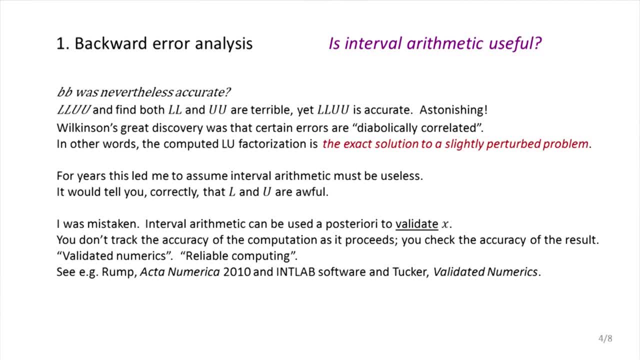 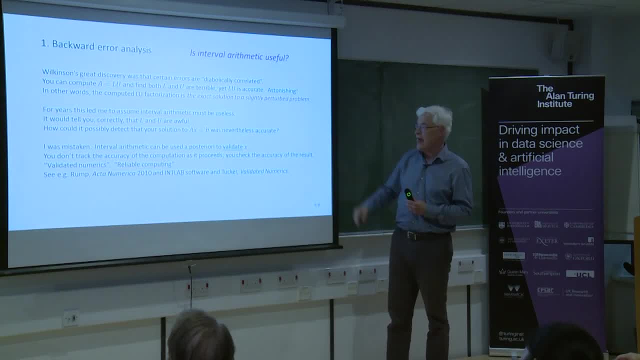 You just take it from an oracle And then you use the interval arithmetic to validate that it's an accurate solution. So you don't track the accuracy. as the computation proceeds, You check the accuracy of the result And this has led to a very successful community. 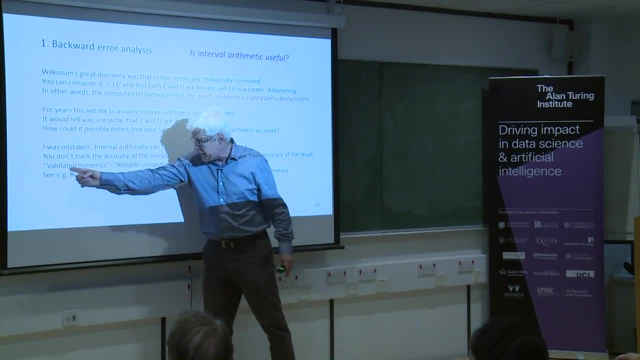 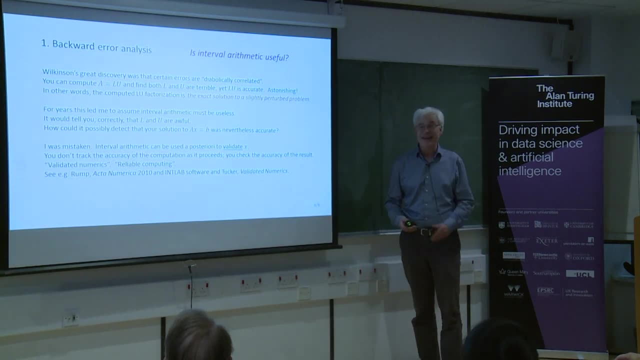 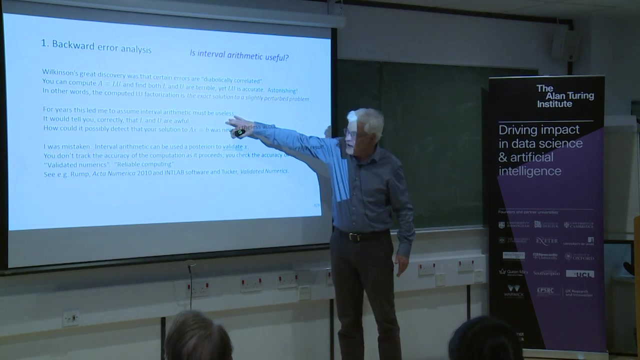 of people who can do remarkable things. There are various phrases: There's validated numerics, There's reliable computing, There's rigorous computing. It's still not at the heart of the computational science enterprise. I still don't think it's something we all need to do all the time. 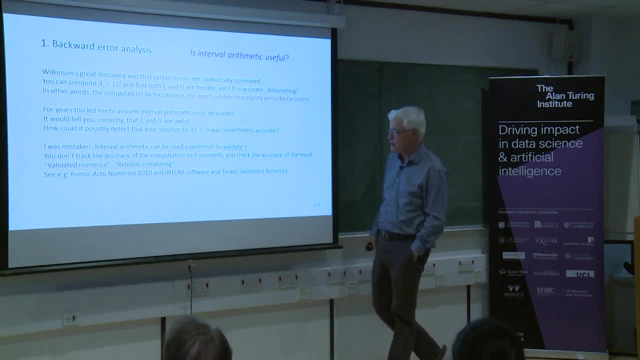 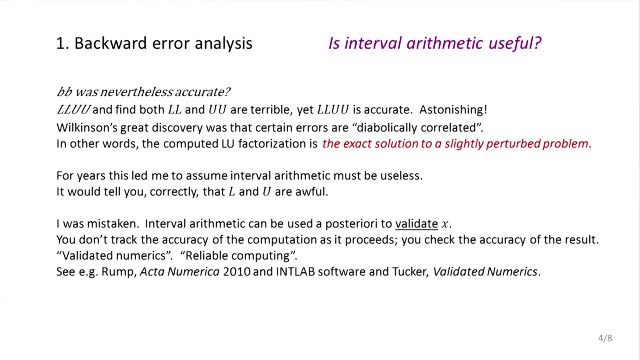 But it's not fundamentally a bad idea. The point is interval. arithmetic is a posteriori. There are many interesting names in this business. Wilfried Rump has this wonderful IntLab software written in Matlab. A predecessor of his was Arnold Neumeier. 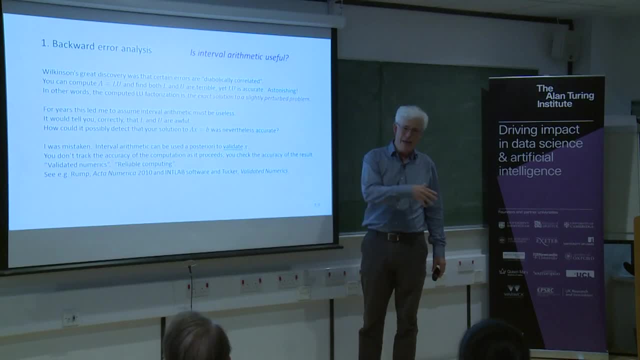 who invented many of these ideas. Even going back to the original book by Moore- this stuff is in there. Warwick Tucker, the guy who proved that the Lorentz attractor exists, has a nice book called Validated Numerics. So I'm just curious. 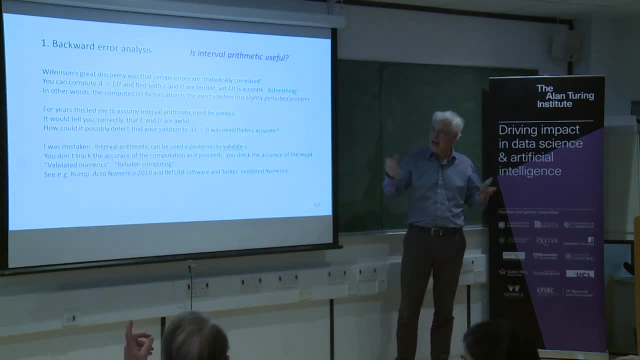 Who has used interval arithmetic. Isn't it amazing how little So it's clearly a kind of a fringe activity. I had a year at INS Lyon where that's what they do- rigorous computing- And I'm persuaded that it's really neat. 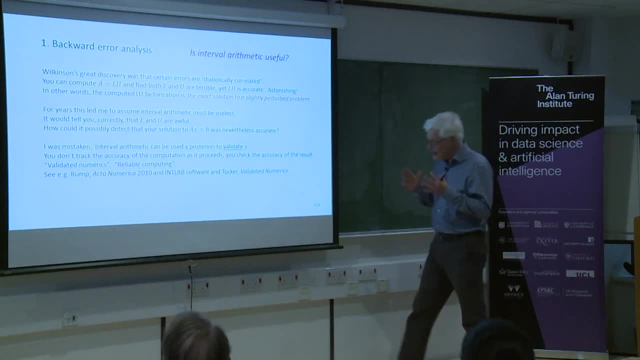 I still don't think you need it most of the time, But I think it's neat and it is a powerful technology. I'm curious to stop for a moment. Any comments on that? Is there anyone else who had the same confusion I did? 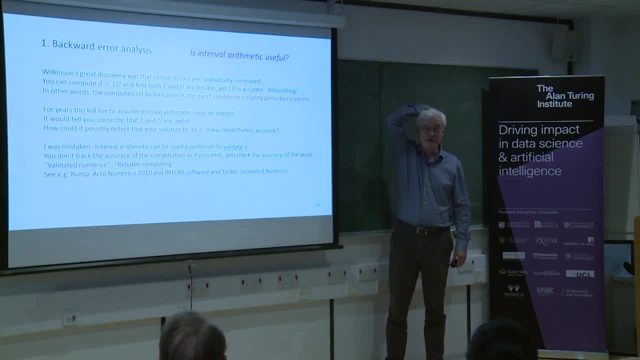 about absorbing Wilkinson and concluding that interval. arithmetic must be a bad idea. Yeah, Uh-huh, Yes, Yeah, I see, Okay, Yeah, Okay. So that's the first of my four points. Now the second one is one that a lot of you know. 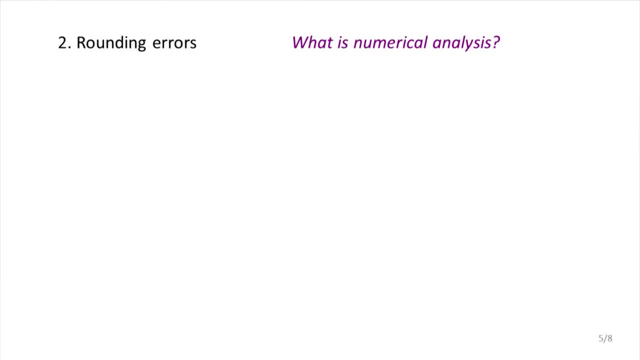 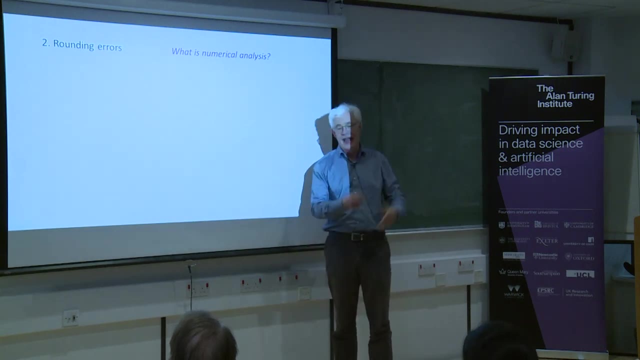 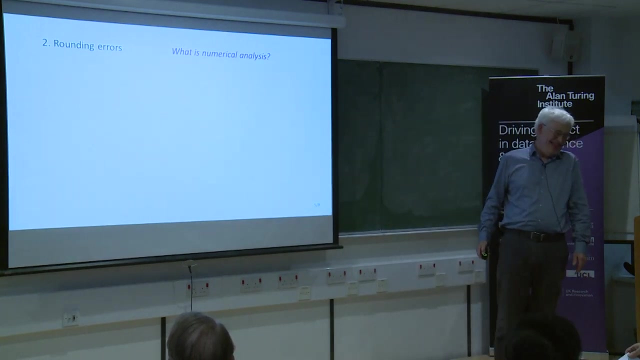 that I bang on about. And here the question I want to relate to is: what is numerical analysis? And, by the way, I don't mean as opposed to scientific computing or something, I mean, what is this subject? we all do? Yes. 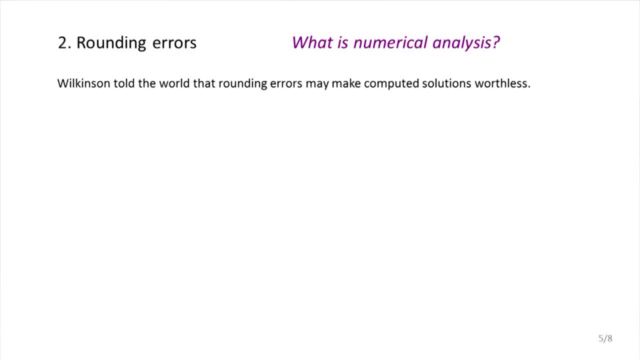 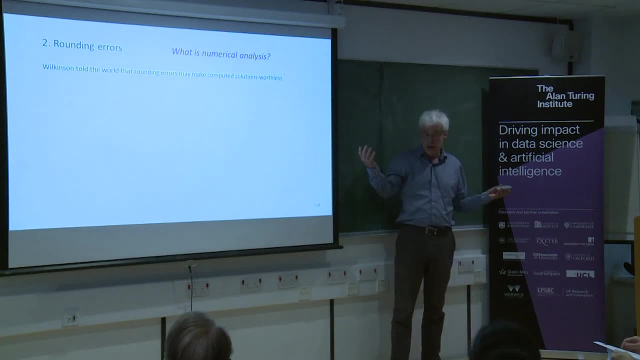 Okay. So Wilkinson told the world that rounding errors may make computed solutions worthless, And I think we've even seen quotes today. This was a shocking discovery to him. He tried to find roots of a polynomial. Out came garbage. This was a big moment for him discovering that. 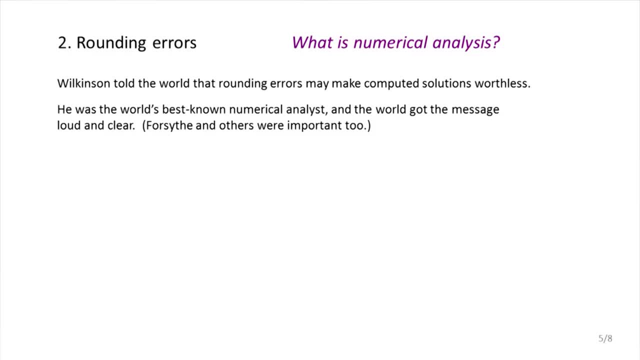 So he was the world's best known numerical analyst, or became that fairly quickly. In the 60s he had that role And the world got the message loud and clear. Wilkinson tells us terrible things can happen when we compute. Now I'm far too young to know the history. 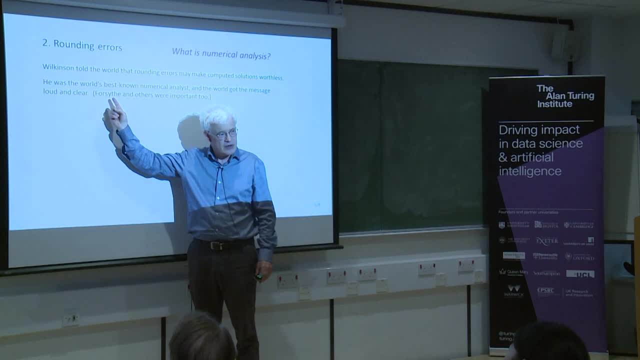 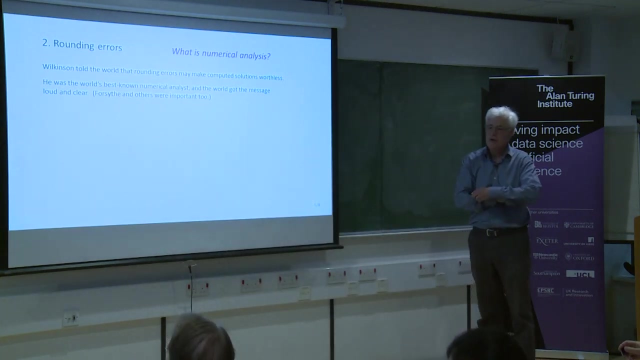 But I think Forsyth was also pretty important in telling the world that, Yeah, You were a young kid but you knew both of them, right? Well, yeah, The first, my first course in numerical analysis at Stanford, the book Rounding Errors and Algebraic Processes. 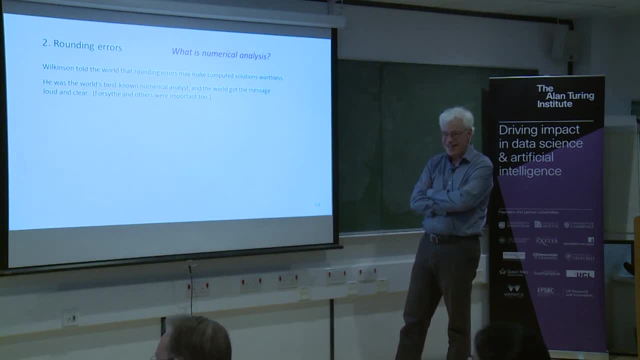 was in preparation, Forsyth was the editor And we read the galley proofs: Yes, In class. Yes, That was our job in class. Yes, Exciting, Well anyway. So Forsyth Wilkinson told the world this discovery. 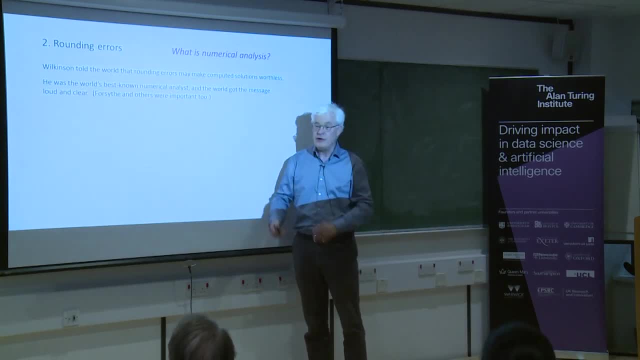 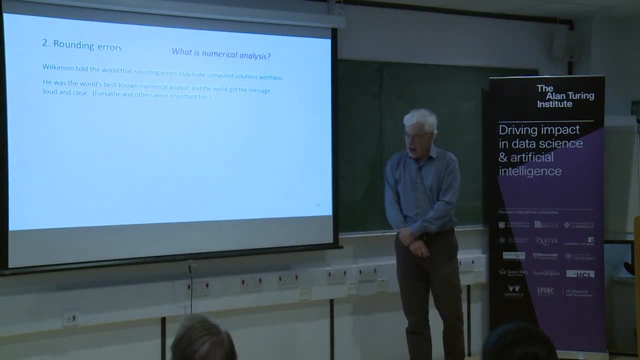 And it's kind of an early 60s discovery And it's kind of an early 60s discovery And it's kind of an early 60s discovery, It's kind of an early 60s era I'm speaking of. 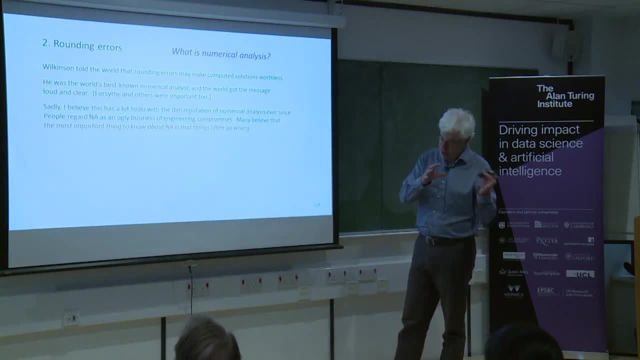 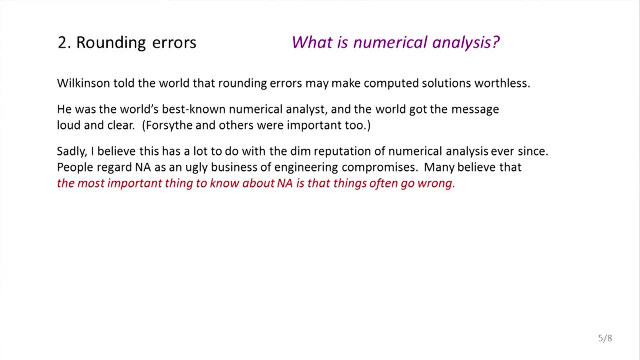 The world really got the message. So, as those of you who've read my essays on the subject know, I think this is a very unfortunate fact of history. I think Wilkinson did as much as anyone to give our field a bad reputation. It's awful. 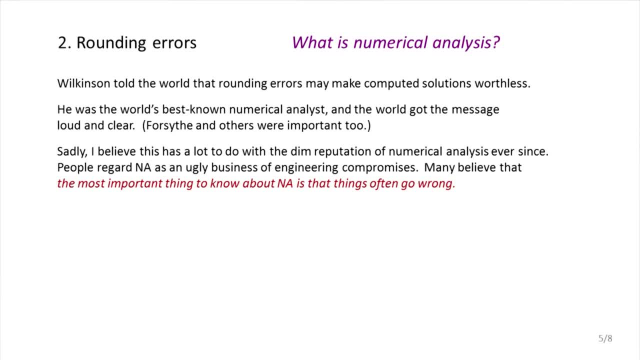 I mean, I don't blame him at the human level. He was doing wonderful, exciting things, But there was this unfortunate effect Numerical analysis has the has a dim reputation. You know, one of my jokes is that mathematicians and computer scientists don't agree on much. 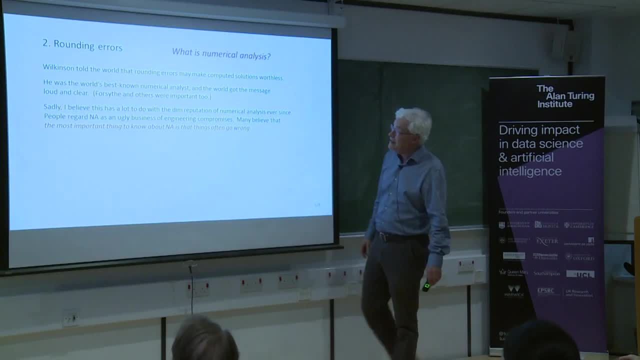 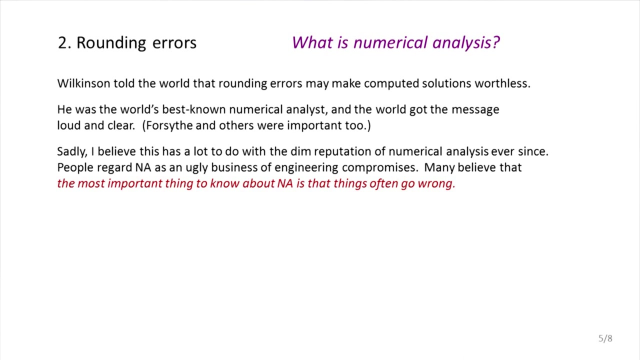 but they agree that this is the worst part of their field. People regard numerical analysis as an ugly story of engineering, compromises, Faustian bargains, And they believe that the most important thing you've got to know about numerical analysis is that things often go wrong. 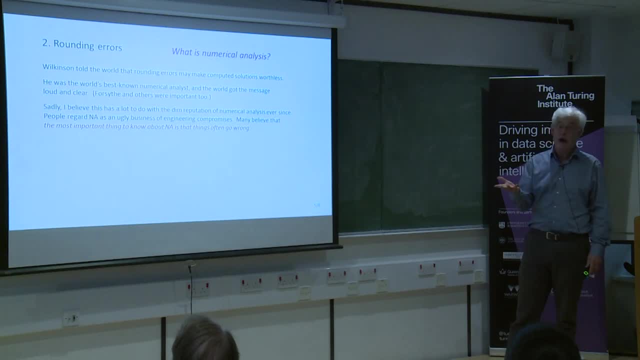 This is a very widespread view, And this has been true throughout my career. actually, Maybe we're being saved a little bit now through data science and suddenly we're coming back in through the back door in a context where accuracy no longer matters anyways. 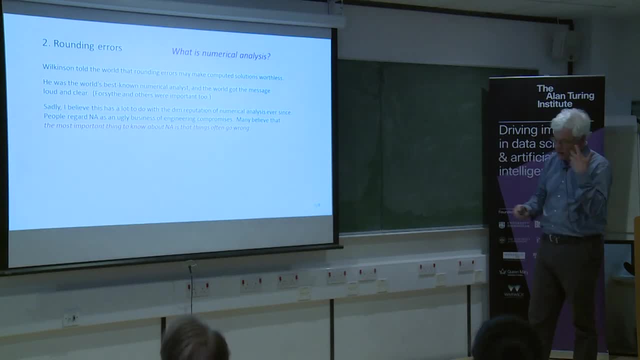 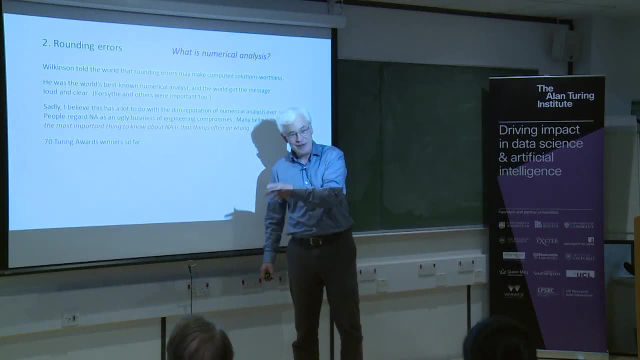 So I think this is an important sad fact that we have to somehow come to grips with those of us in this field. Let me make a remark about Turing Awards. I just was looking this up on the web this morning. So there have been 70 Turing Award winners so far. 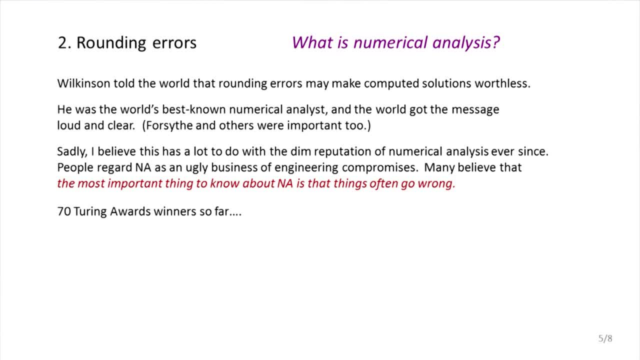 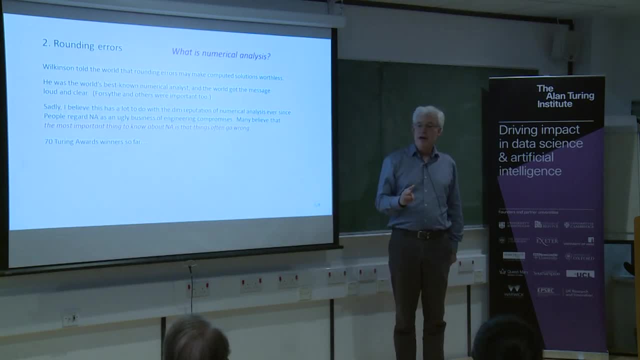 I think 53 events, But some of them are double. Who can name some numerical analysts? Cahan, Cahan, Wilkinson, Wilkinson, That's all. Well, there's two and a half, So the other one would be Hamming. 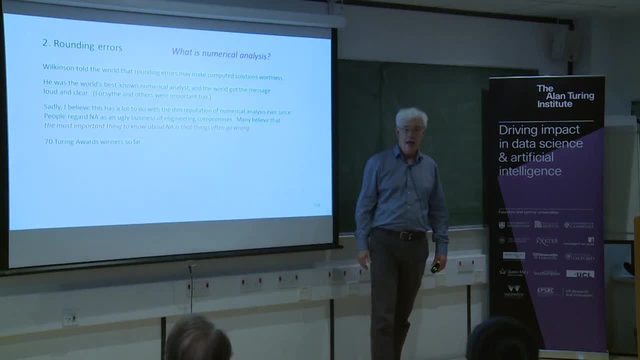 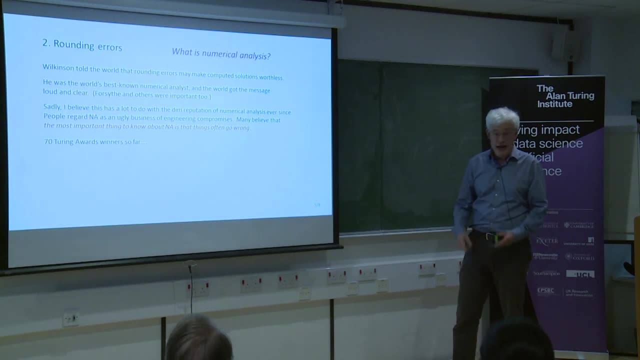 Now, mostly he was known for coding. Yeah, But so, and now when I've looked online, you know what are these guys praised for when they get their Turing Award. It's error analysis. So first you have Wilkinson back in 1970.. 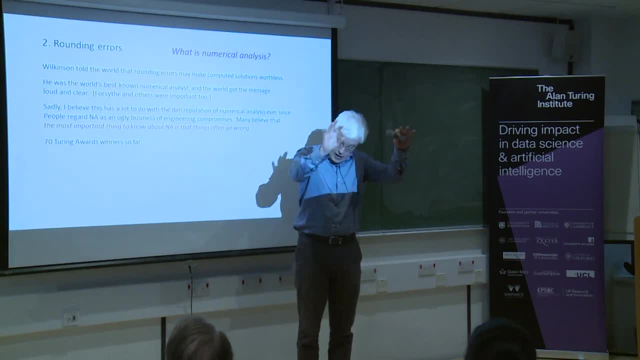 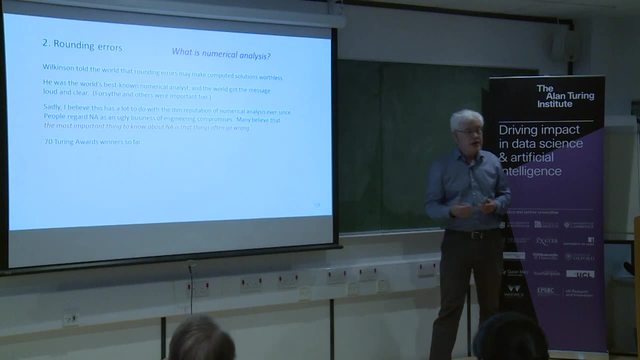 Whenever. And of course the citation mentions linear algebra, but it mentions that he gave us backward error analysis. And then Cahan, of course it's floating point arithmetic. You know the fact that Cahan is a great genius of numerical linear algebra. 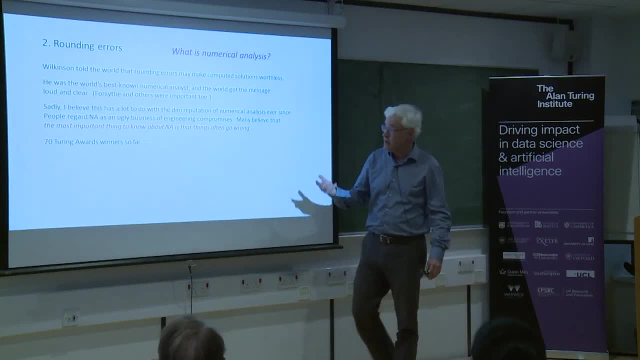 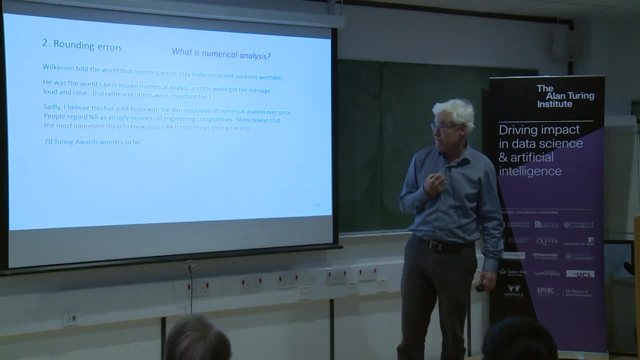 that didn't interest the Turing Committee. No, it was floating point, arithmetic, of course. So if you look at the Turing Awards, that backs up this hypothesis that computer scientists perceive our field as the study of errors. Now what about the ratio three over 70?? 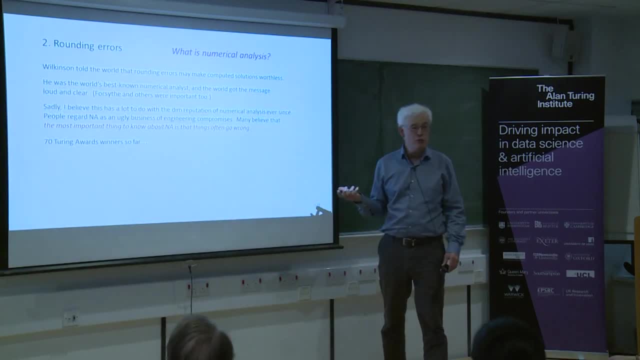 So back in the 60s, computer science departments were founded in almost every case by an alliance between a couple of numerical people and a couple of non-numerical people. at places like Michigan or Stanford or Oxford, You always you know it was a half-numerical subject. 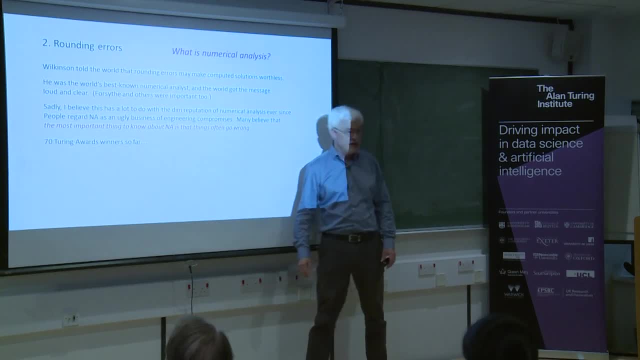 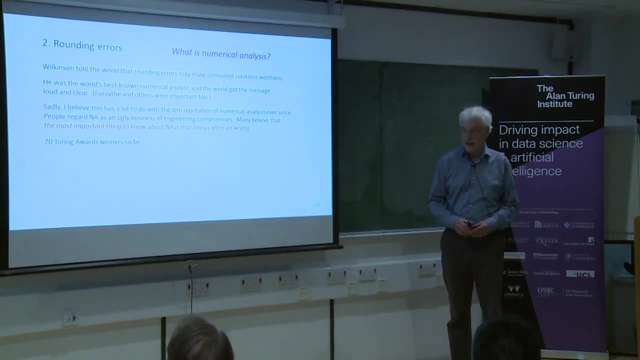 being created in the academic world in the 60s. Anyone in the 60s would have said that numerical analysis was a half or a third or something of computer science. Well, it's three-seventieths of computer science, according to the Turing Award calculation. 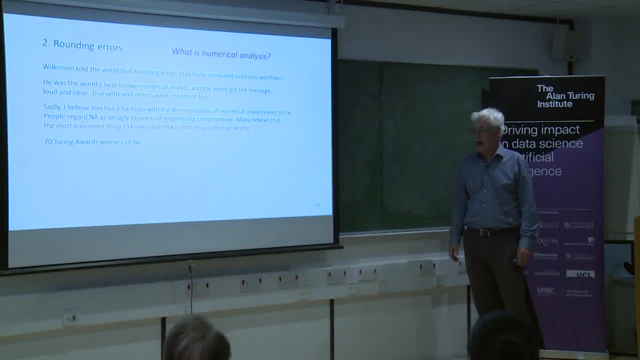 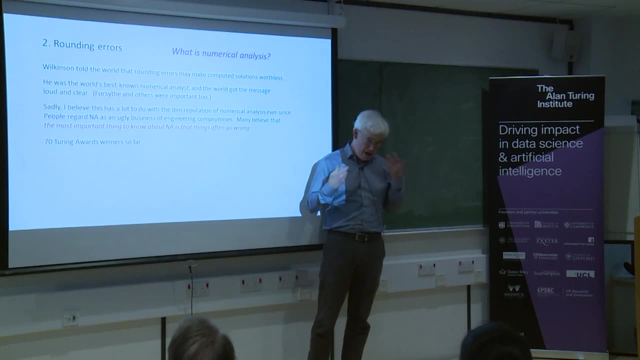 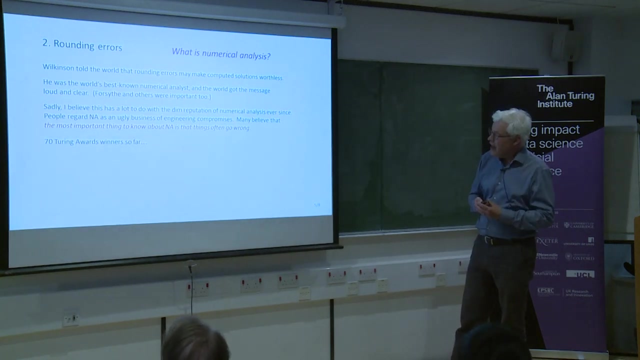 I'm not saying that I believe it should be half- I don't- But I am saying that this is yet another reflection. that low number is another reflection of the weird state that our field is in reputationally, which sadly has something to do with my hero. 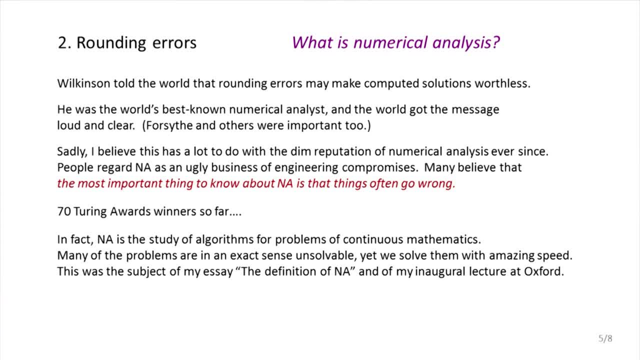 So, in fact, the right definition is that it's the study of algorithms for the problems of continuous mathematics. The rest of computer science is the study of algorithms for the problems of discrete mathematics And, as you know, if you've read my stuff, 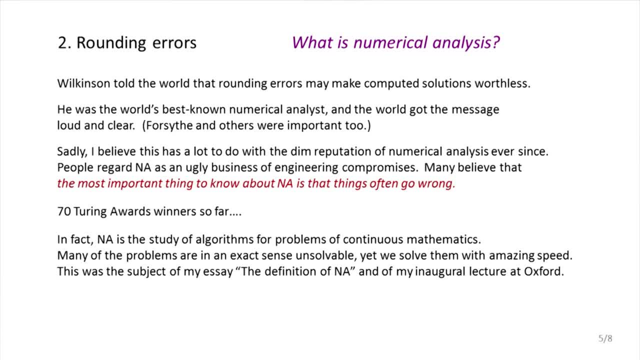 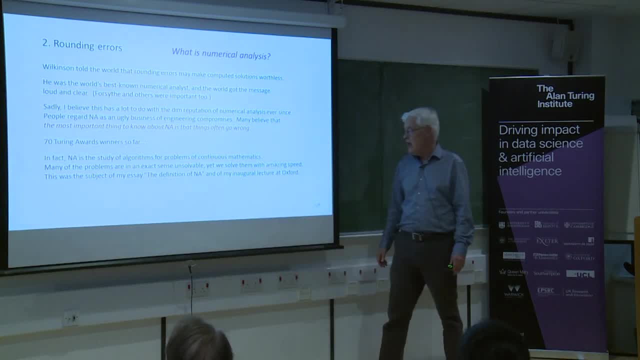 I think the great drama of numerical analysis is that we solve problems that in principle can't be solved. There's no analytic solution very often And we solve them with incredible speed. Or sometimes they can be solved, but in n-cubed operations. 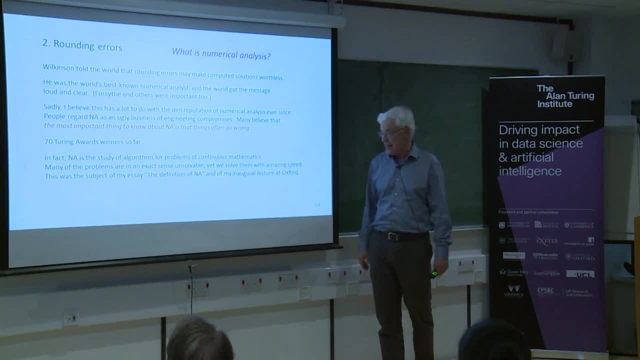 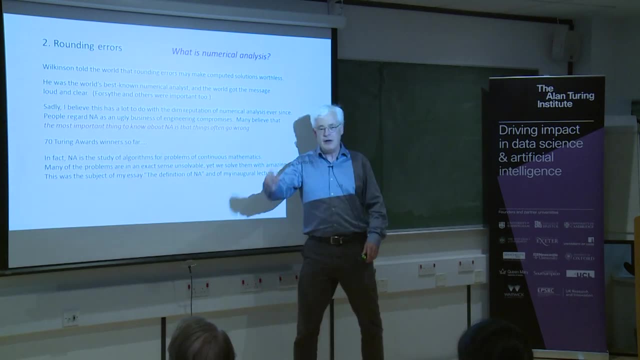 and we find a way to do it better. We can do it in n-squared or n-log n. That's amazing and it fundamentally had little to do with error analysis. So raise your hand. if you've read that essay, I'm curious. 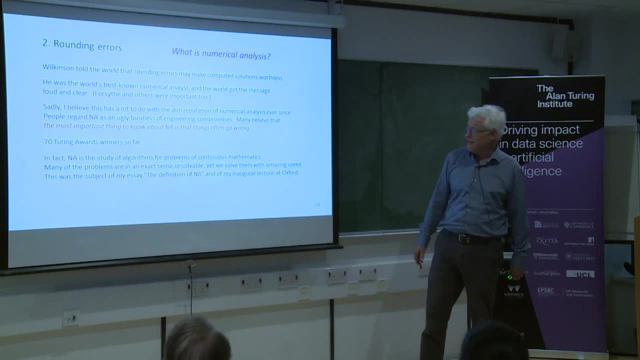 Actually I expected even more, because it's a great essay. Okay, Oh, I wanted to tell two stories. So they're 25 years apart And these are two wonderful people. I'm sure many of you know David Gries at Cornell. 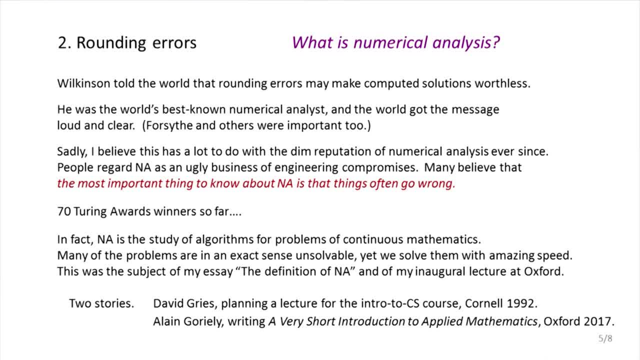 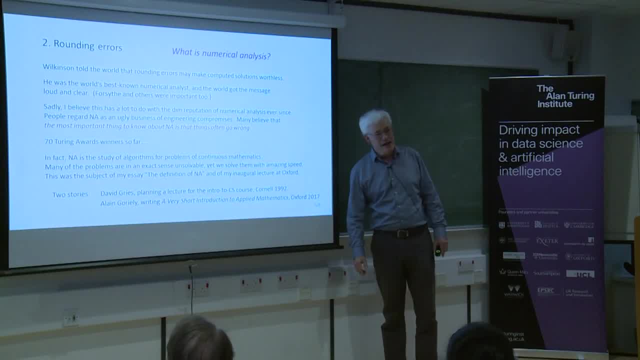 Fantastic guy, Alain Gorielli, the professor of applied mathematics at Oxford, Also wonderful. These are great people. So I remember when I was at Cornell, David came into my office. He was teaching, you know, CS 101.. 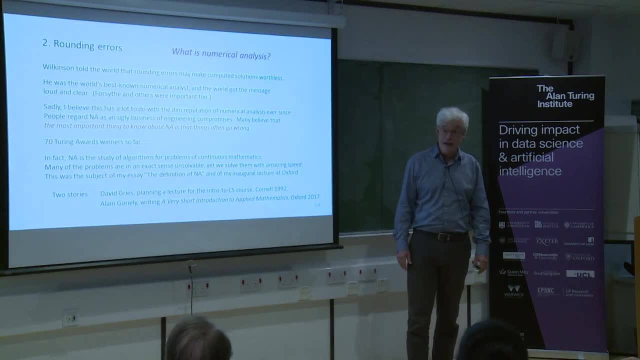 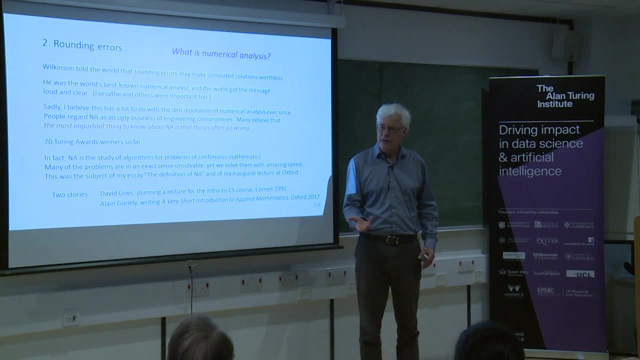 And he said: tomorrow I have to give a lecture on numerical analysis. Now I know that the main thing I have to tell him is that these methods don't work, But can you give me a good example? So it was incredible. Yeah, I cried. 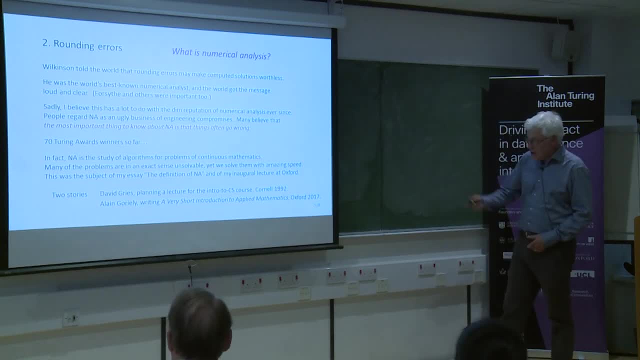 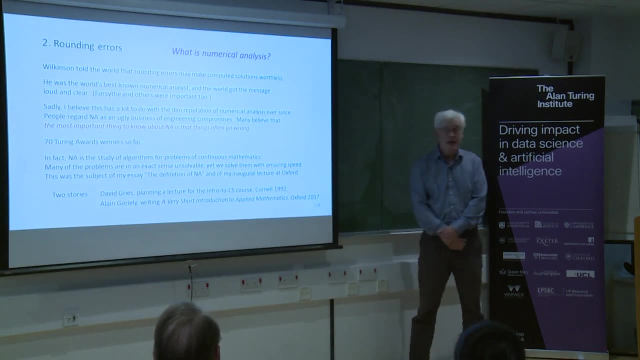 I yelled. Twenty-five years later. you all know the series of very short introductions, and Alain was writing the one on applied mathematics. Now, applied mathematics, as you know, has the modeling side, which is close to the natural world. 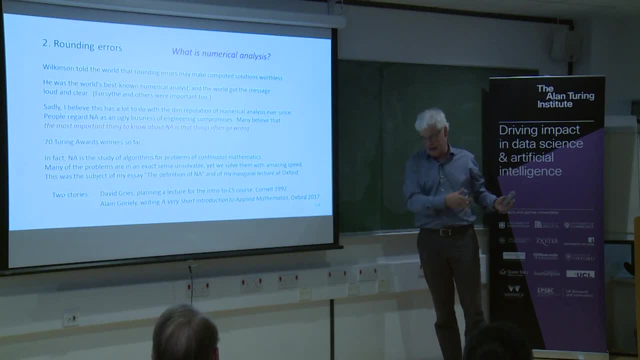 and then it has the algorithms. mathematical side rather different. I'm very much on the algorithm side, but at Oxford most would be on the modeling side and that would surely be the bigger half of applied mathematics. So I read his whole draft. 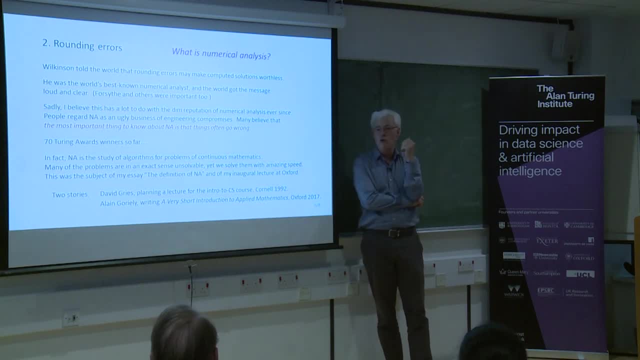 and in these hundred pages or so there were four or five pages on numerical analysis. And guess what? The central message was that it often gave you the wrong answer. There was one plot in these pages and it had two curves, and one of them was labeled numerical solution. 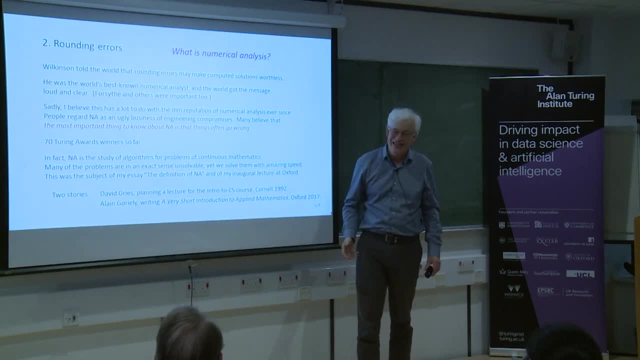 and the point of the figure was that it was wrong. I mean, you know, I can't even finish my sentence. I can't even start the sentence. It's not that he's wickedly trying to do us down, Of course not. 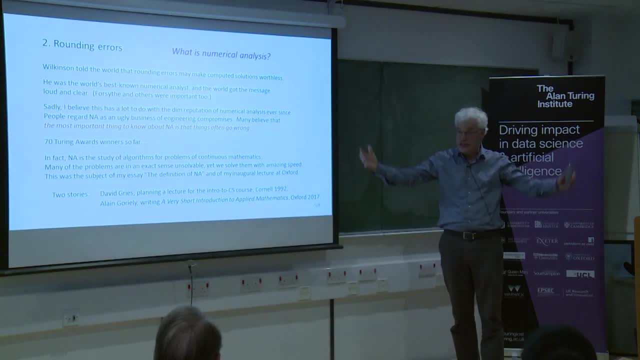 It's that people don't see the huge fact, which is that all the time we're getting correct answers from all sorts of problems. they focus on the small fact, which is that you've got to be careful. More say you write essays about how numerical analysis go wrong. 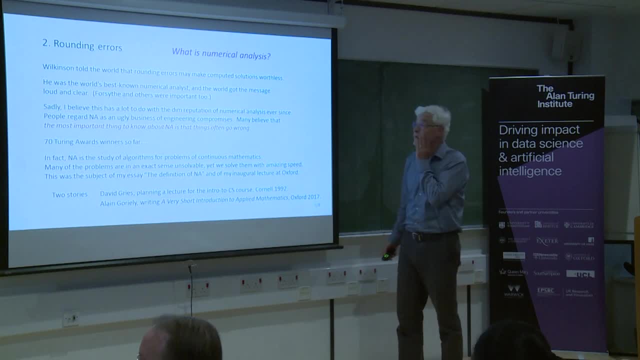 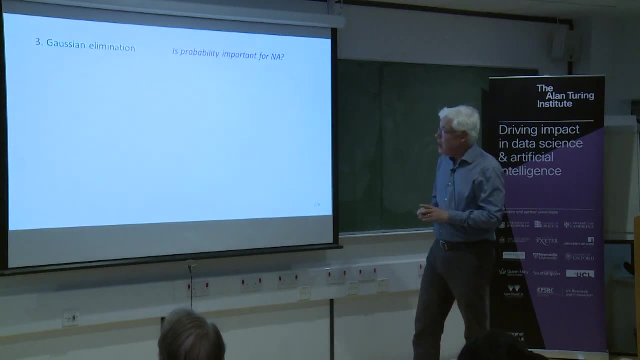 Uh-huh, Only the quadratic. Yes, I read that essay. Yeah, Whatever there's something about, whatever mathematician should know about it. Yep, yep, yep. The third topic has already come up in the last talk. 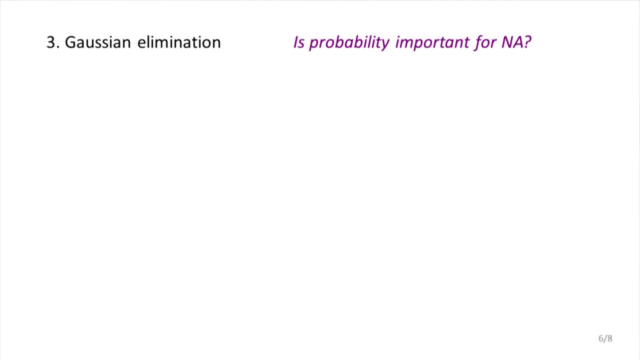 even Gaussian elimination, and I want to relate that to probability. So, as we know, one of Wilkinson's triumphs was his analysis of Gaussian elimination, the big paper from 1961. It had been predicted by some obscure people that exponential growth of errors was a problem. 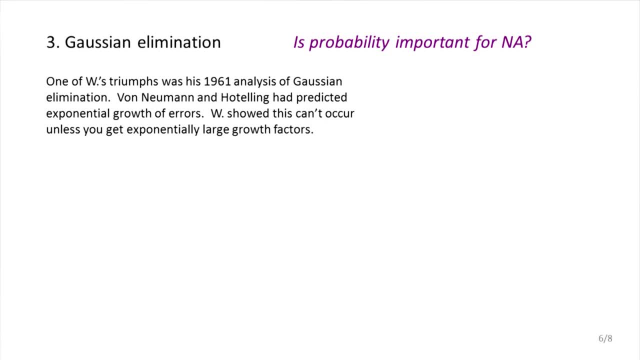 and Wilkinson rigorously proved that this can't happen. Well, unless you get large growth factors. The trouble is, you can get large growth factors. So, formally speaking, Wilkinson did not show anything about the stability of Gaussian elimination, except that it had to take a certain form. 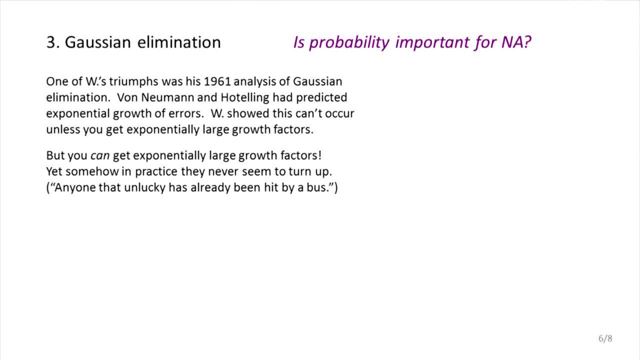 But he didn't show it won't occur. And people say things like somehow in practice they never seem to turn up. you know, as if this requires some weird explanation. I'm not sure if Wilkinson said this, but certainly it's an urban myth. 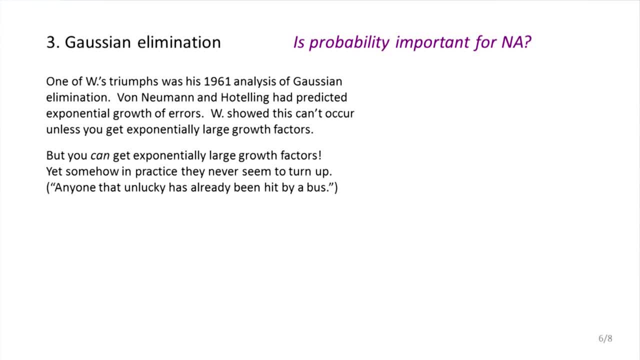 that Wilkinson said. anyone that unlucky has already been hit by a bus. Anyway, there's nothing magical going on, It's all about probability, And I've been saying this for many years, but nobody's really interested. So the explanation is probabilistic. 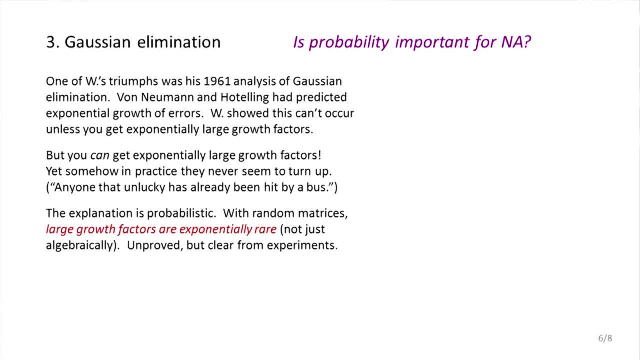 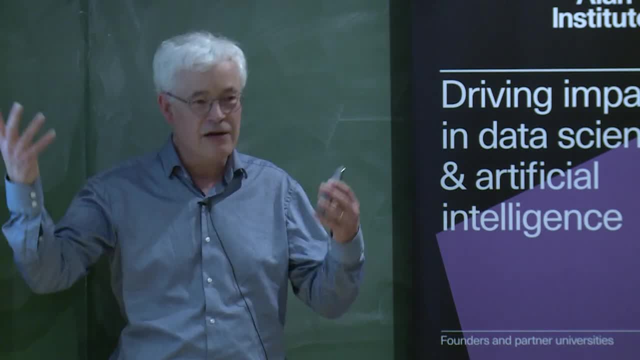 It has not yet been proved, but let me show you data which makes it overwhelmingly clear. Suppose you take random matrices, and it's much the same with any distribution, but here of course we take independent Gaussian entries. And suppose you take these random matrices. 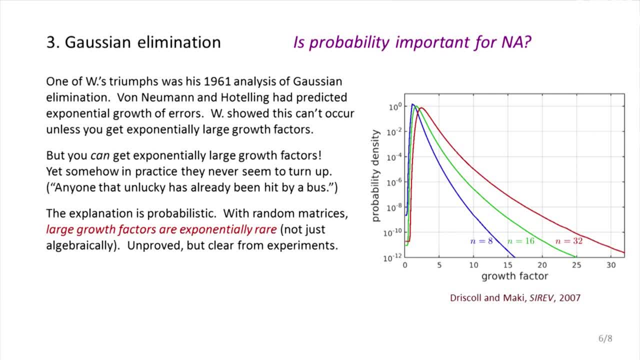 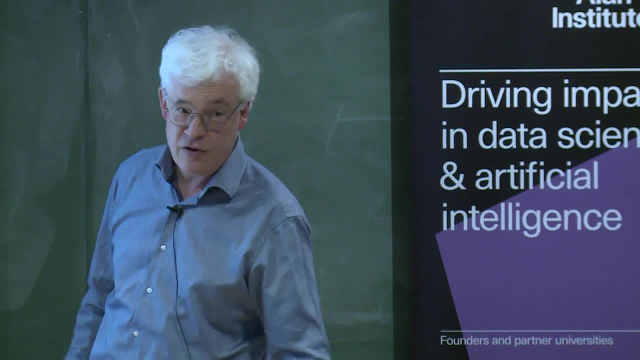 and look at their growth factors for Gaussian elimination with partial pivoting. These are probability distributions for 8 by 8,, 16 by 16, and 32 by 32.. And the thing is, notice the log scale here. So the probability with an 8 by 8,. 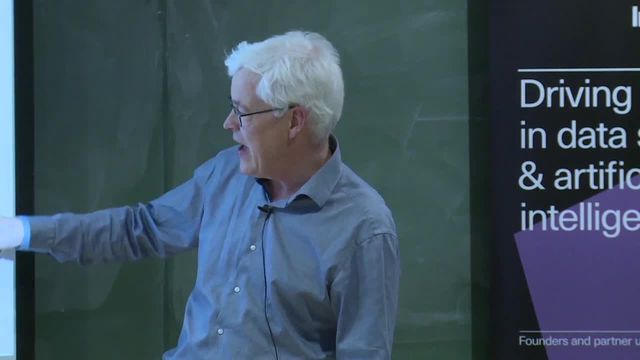 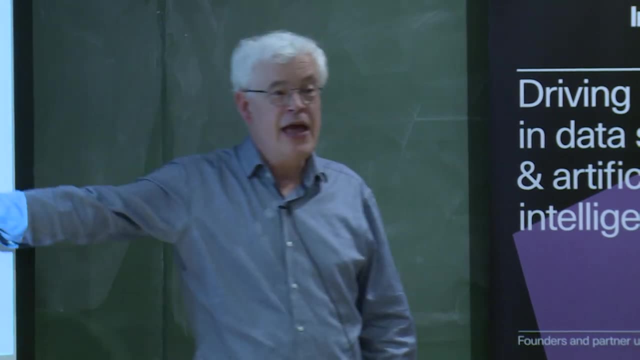 well, 32 by 32, matrix of getting a growth factor of 25 is 10 to the minus tenth. So this is not algebraic decay, This is exponential or root exponential decay We're getting. There's some exponential phenomenon going on. 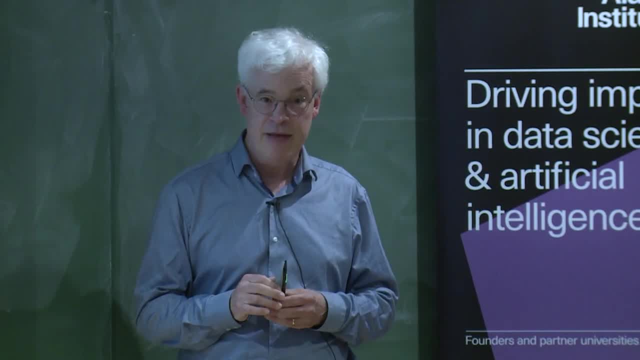 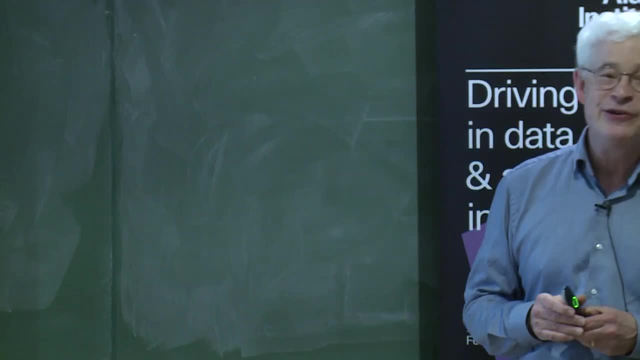 that makes partial pivoting spectacularly stable. Now, given that this is the most successful numerical algorithm of all time, you would think that there would be a literature on this subject, but there isn't. Nobody's interested. Nobody has attempted to fix this. 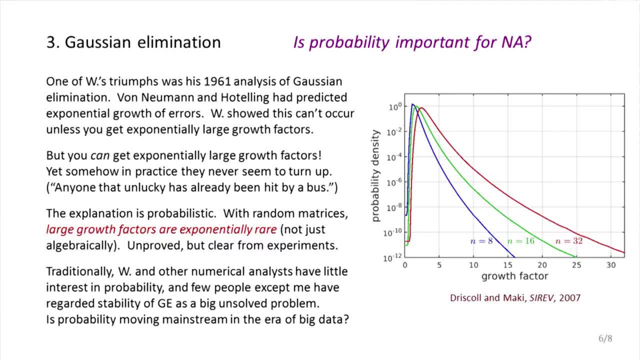 or to explain it, except me, and I've failed. These beautiful computations come from Toby Driscoll and Karamaki. It's not. They had to do fancy stuff to get such accuracy. So there's an incredible phenomenon there of exponentially small probabilities. 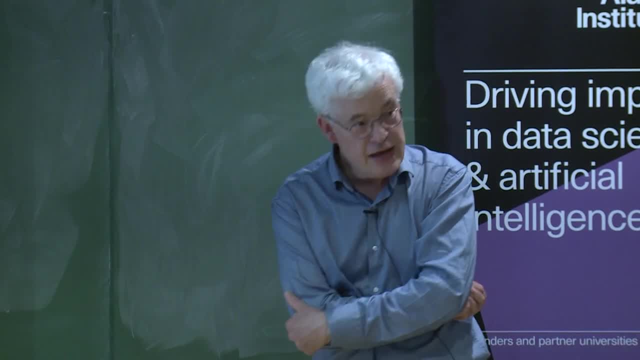 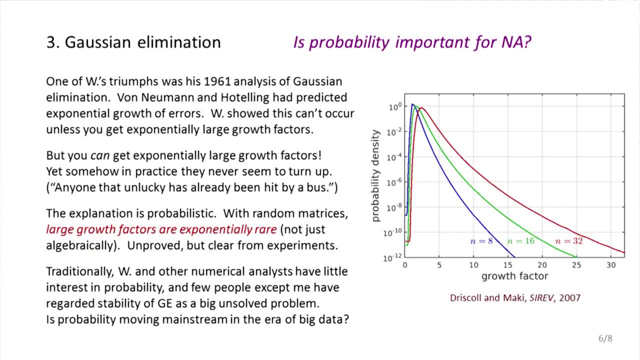 waiting to be explained, I think. in fact the mathematics is. The explanation is close to compressed sensing. So we're entering an era when things may be changing. Wilkinson really wasn't interested in probability. He I don't know why this effect interested him. 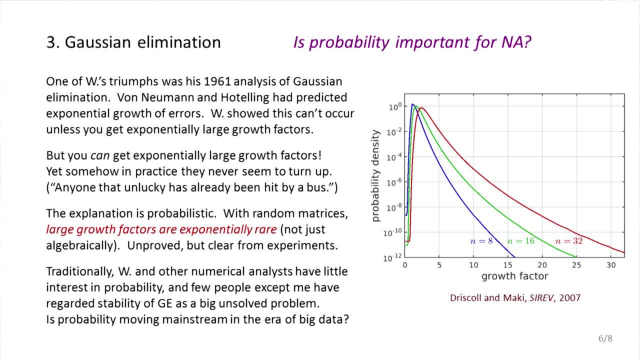 It interested him so little. I wouldn't be surprised if he tried to prove something and failed and then pushed it aside because it's so striking. But he doesn't discuss that. He didn't talk about probability. in this sense, Very few people have paid any attention to this problem. 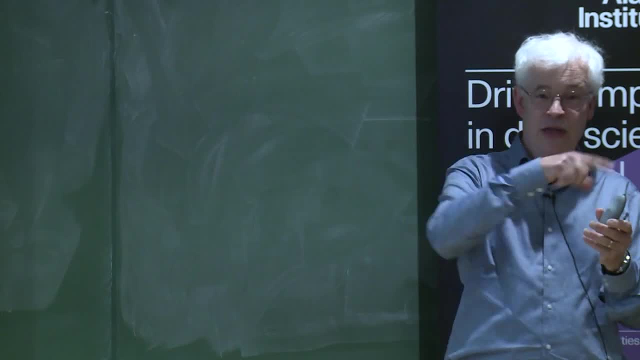 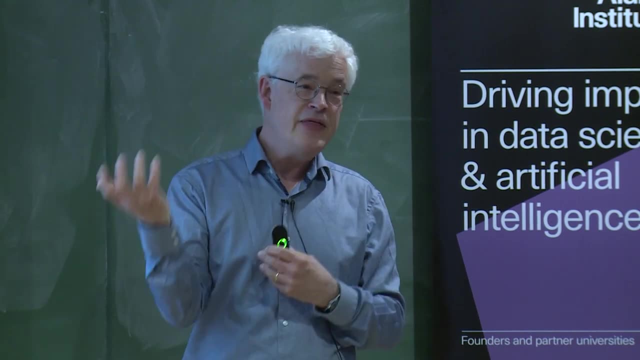 But I think things are changing. So the whole field of compressed sensing is all about these phase transitions and it's always exponential effects going on In computer science, like cryptology, all of the things you do to get nearly perfect communication between Alice and Bob. 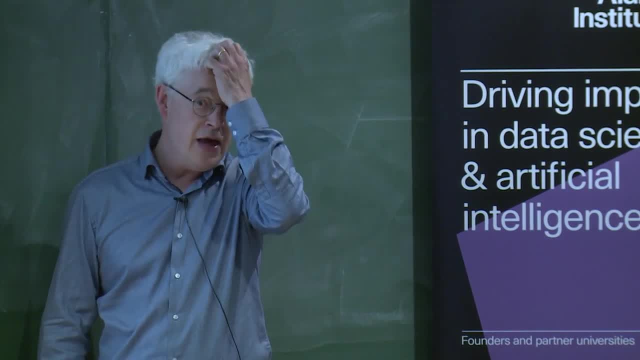 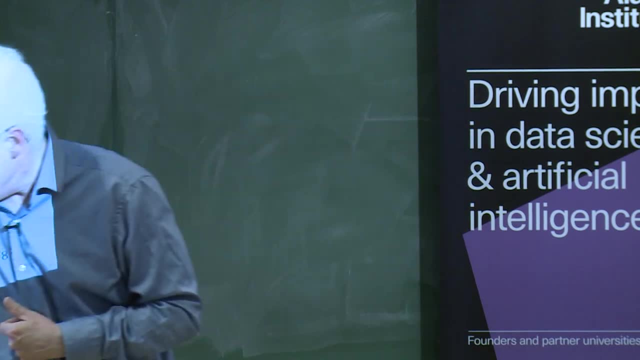 it's always exponential. Algebraic is never good enough. Exponential Probabilistic algorithms with exponential effects are the ones we rely on all the time. So I think maybe at last we're going to solve this problem and spring numerical analysis. 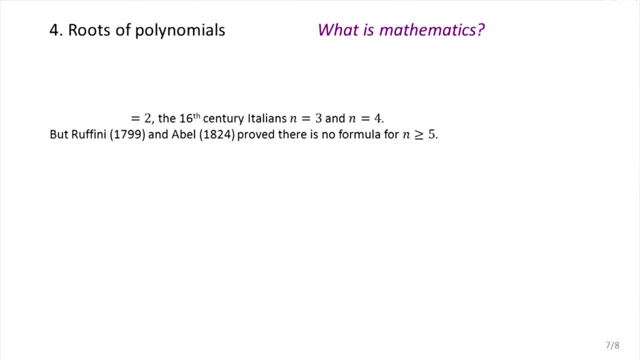 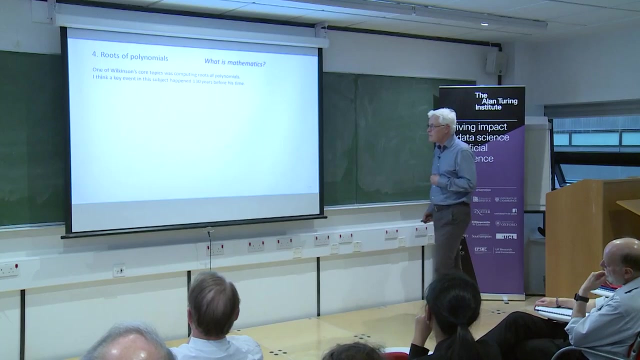 a little closer to other subjects. The fourth topic is roots of polynomials, with lovable subjects, And my modest ambition there is to have it shed light on the question of what is mathematics. So, as we know, Wilkinson was very interested in this subject. 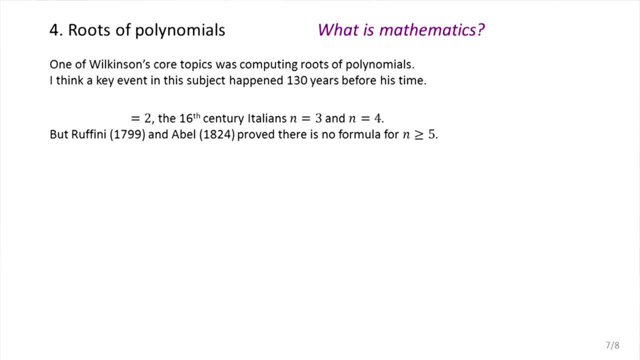 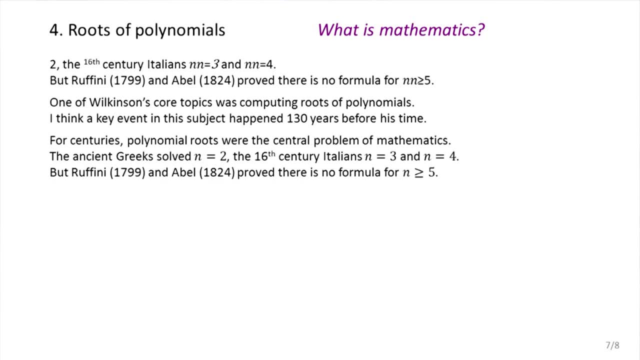 And I think something very important happened 130 years before. he was working on roots of polynomials. So essentially, root finding was the central problem of mathematics in the Middle Ages The Greeks had done the quadratic case, but then the Italians managed to do. 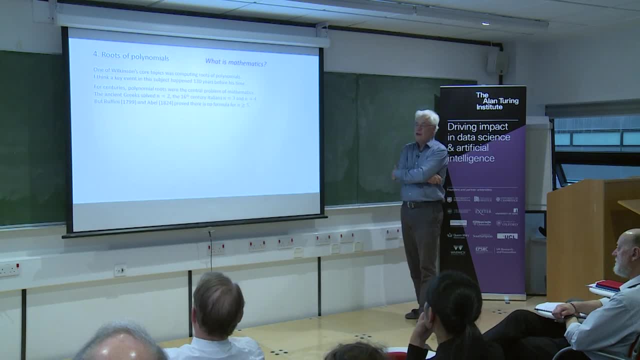 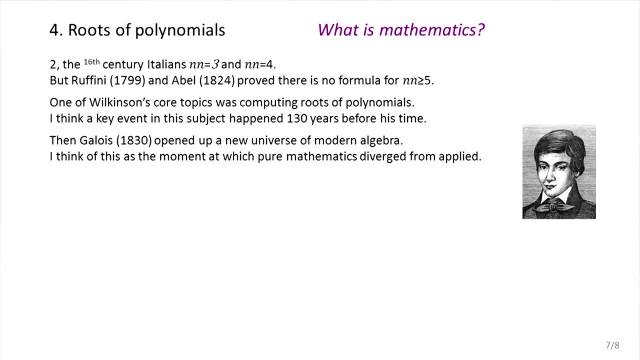 degree three and degree four. But then it was proved that you couldn't do quintics and above in the standard sense. And then this guy Galois, who we all know about, wrote a couple of amazing papers. It took a while for them to have impact. 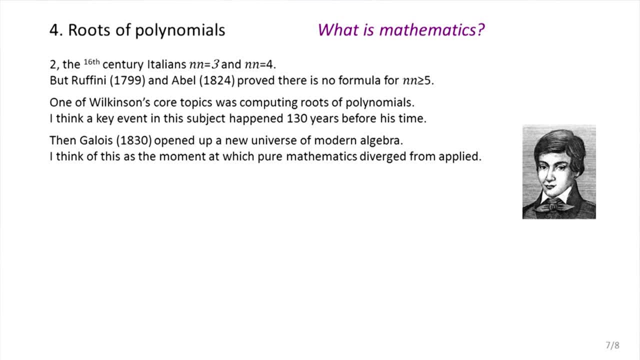 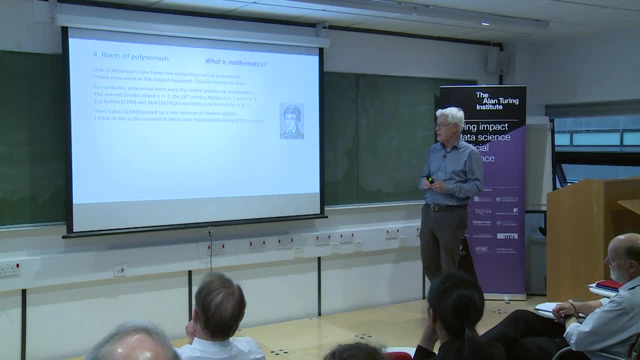 but eventually their impact was extraordinary. They changed everything. I think of Galois as the moment at which pure and applied mathematics diverged. And let me explain. I'm guessing none of you know Galois. You know Galois theory very well. 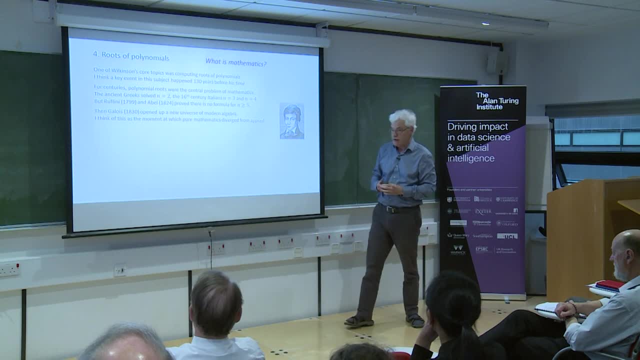 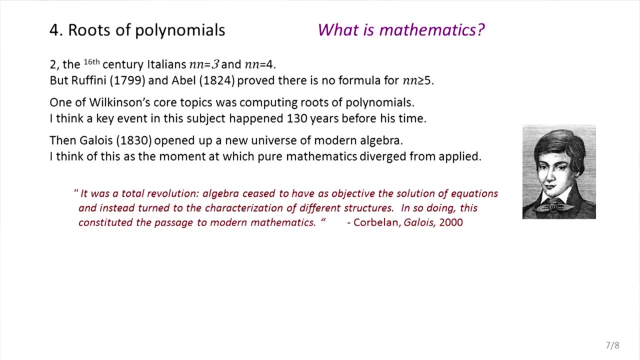 and I certainly don't, But it's a beautiful subject, which involves algebraic structures that are connected with roots of polynomials. I read a biography of Galois last year and here's one of many similar quotes about what he did. It was a total revolution. 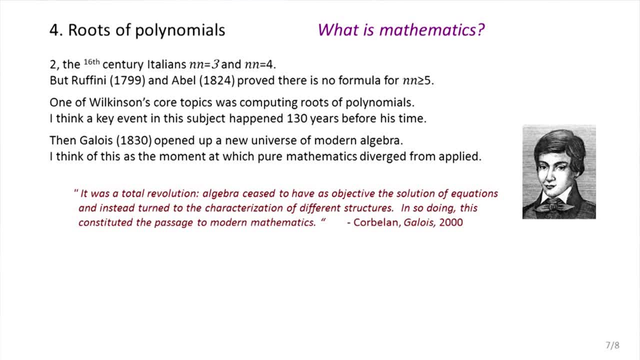 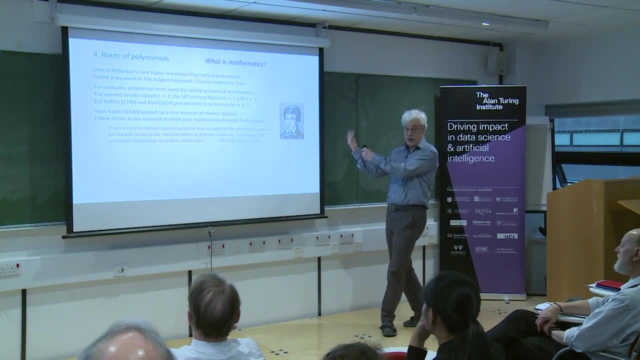 Algebra seeks to have as objective the solution of equations and instead turn to the characterization of different structures. In so doing, this constituted the passage to modern mathematics. Well, it's an incredible statement. Think what that's saying, You know he discovered something new. 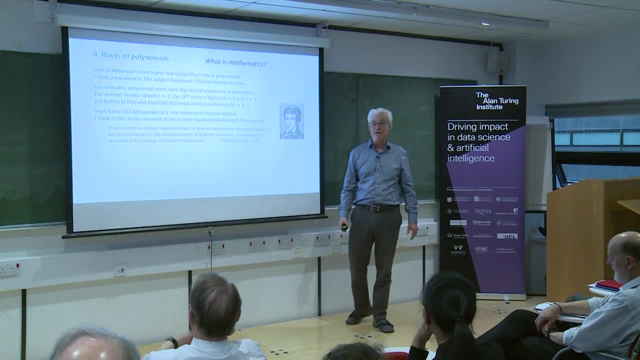 Well, what about the old problem? It's not as if he solved it. He merely said: I've got another problem to distract you with right. So did root finding cease to be important in 1830?? Of course not. 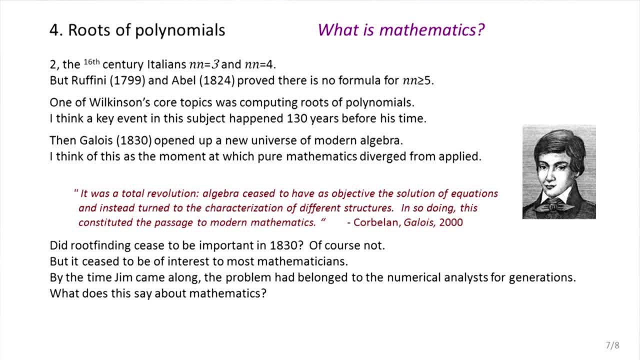 but it ceased to be of interest to most mathematicians And by the time Jim came along, no respectable mathematician would even dream of talking about algorithms for root finding. So what does that say about the connection of mathematics to the scientific world? You know? 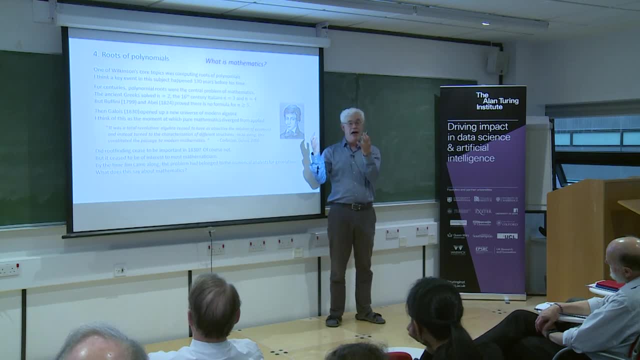 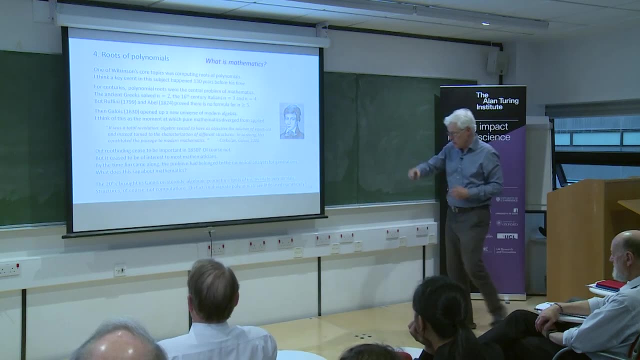 that a problem like this ceases even to be one that real mathematicians perceive when they look at the mathematical universe. Oh so the 20.. I hate the steroids word- We've had it twice now- But anyway, in the 20th century. 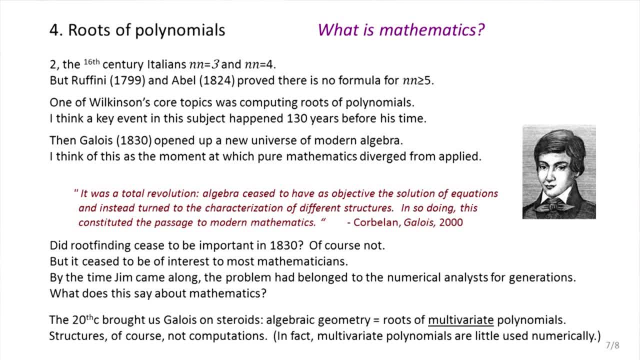 everything went up a notch with algebraic geometry, which is the heart of pure mathematics. It's all about structures associated with roots of multivariate polynomials, Further and further from things that people like us really care about. Okay, so I One minute, I guess. 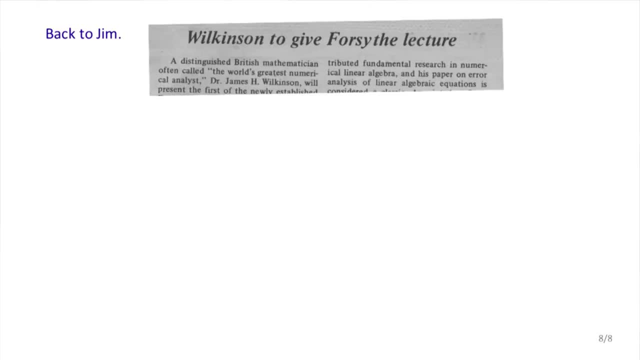 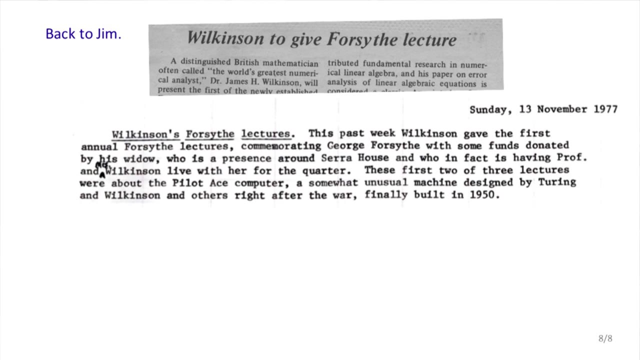 I'll finish up. So back to Jim. While I was there he gave a sequence of Forsyth lectures and here are my diary notes. This past week Wilkinson gave the first annual Forsyth lectures, commemorating Forsyth with some funds. 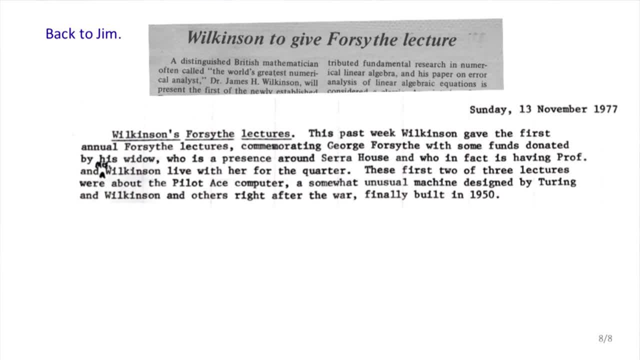 donated by his widow, who is a presence around Serra House and who, in fact, is having Professor and Mrs Wilkinson live with her for the quarter. These first two of the lectures were written by. these first two of three lectures were about the Pilot Ace computer. 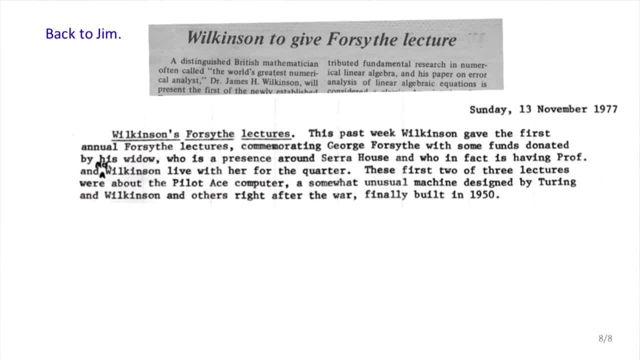 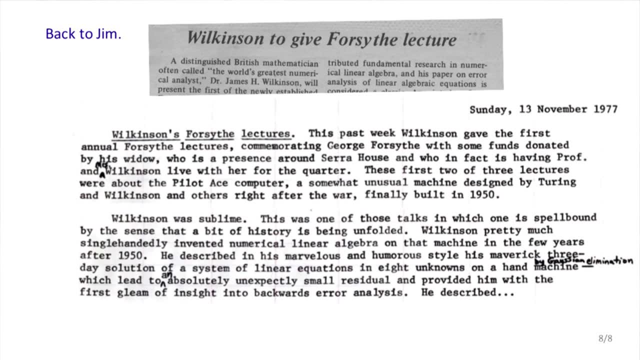 a somewhat unusual machine designed by Turing and Wilkinson and others right after the war, finally built in 1950.. Wilkinson was sublime. This was one of those talks in which one is spellbound by the sense that a bit of history is being unfolded. 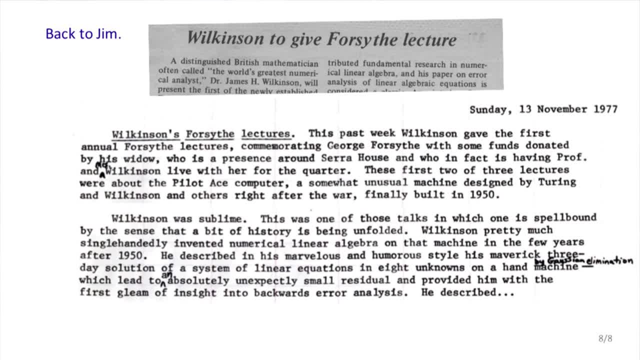 Wilkinson pretty much single-handedly invented numerical linear algebra on that machine in the few years after 1950.. He described in his marvelous and humorous style his maverick three-day solution of a system of linear equations and unknowns on a hand machine by Gaussian elimination. 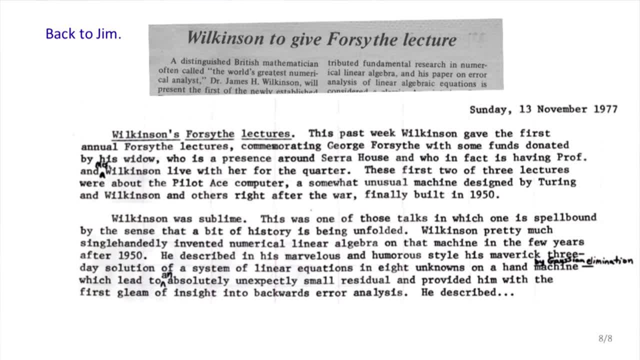 which led to an absolutely unexpectedly small residual and provided him with the first gleam of insight into backwards error analysis He described: these are my dots from then and then the final line is: these were two great lectures. Wilkinson is a delight to everyone. 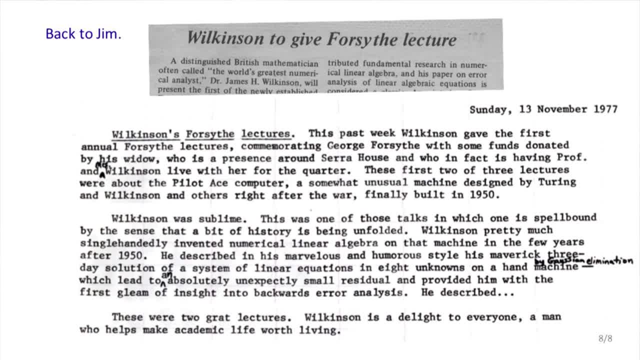 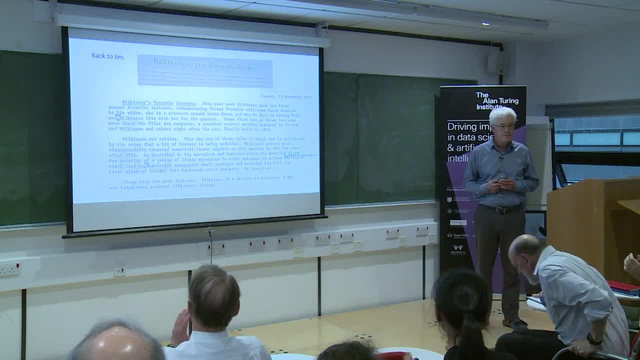 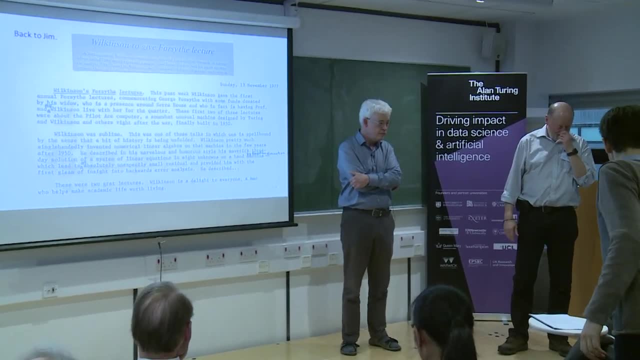 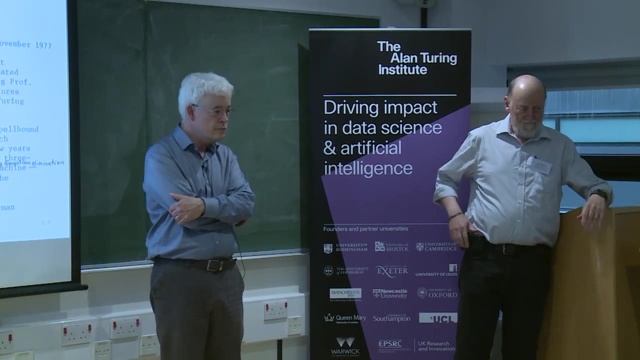 a man who helps make academic life worth living. So thank you. I think it's only fair to point out it was Harald Hotling who predicted the four to the n growth in Gaussian elimination. I don't think von Neumann ever did that. 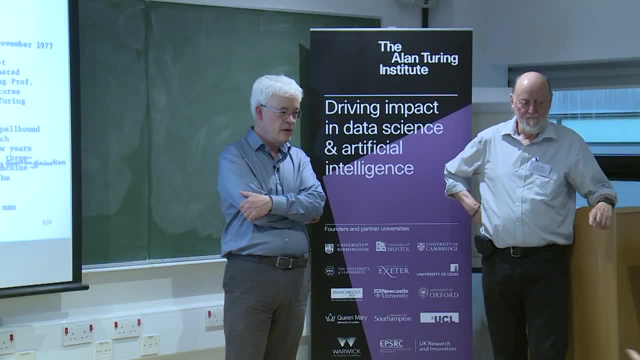 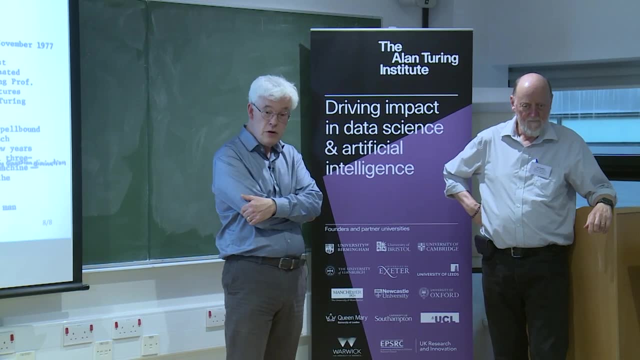 I think he had two to the n. He had the error analysis, that long error analysis that That led to two to the n, didn't it? No, No, No, Okay. It showed stability or positive definite system, Okay. 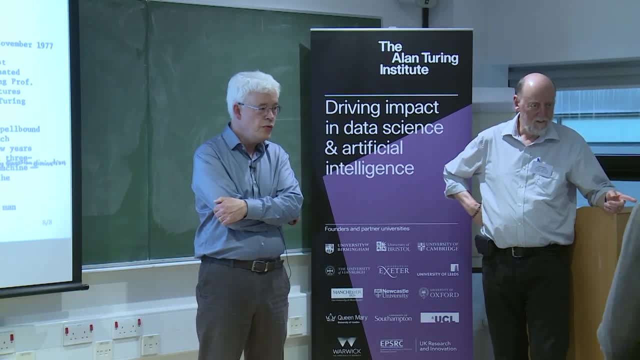 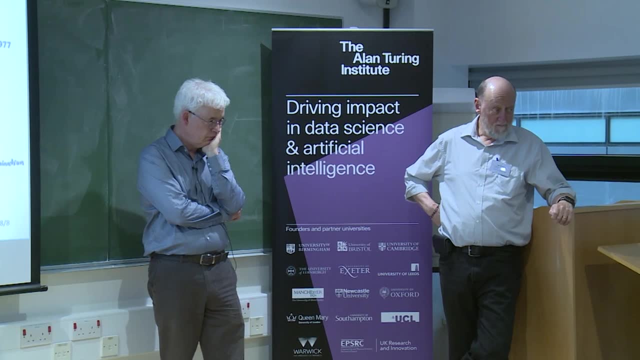 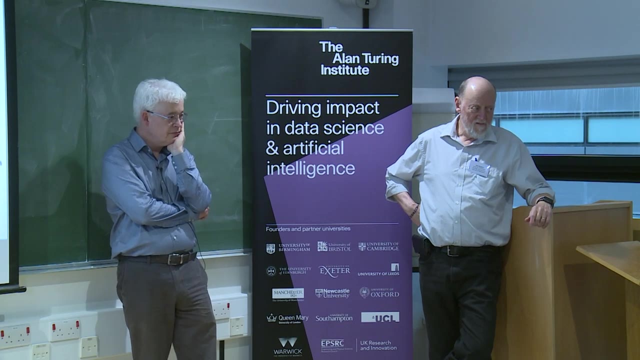 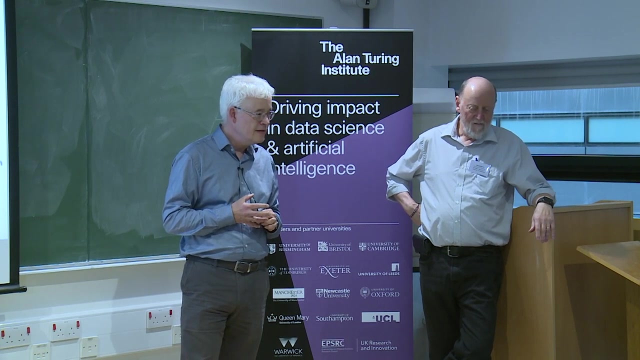 Yeah, I think you're perfectly right that the message that we're giving, that we're warning that things could go wrong, are always misinterpreted in the sense of that usually everything goes wrong. This, I think, is a message that is mistaken. 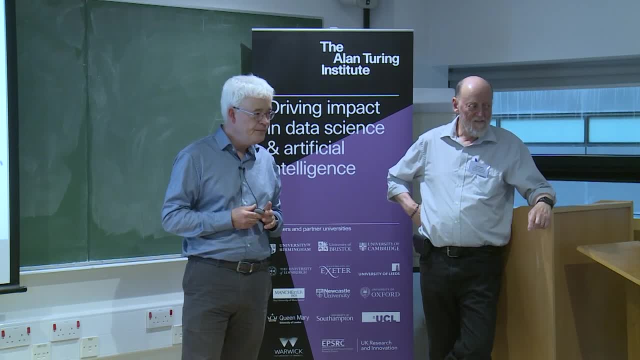 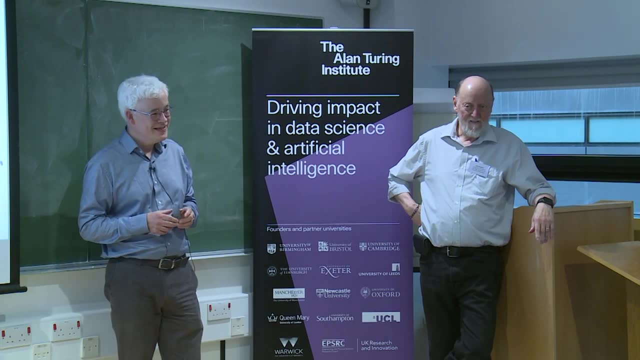 from the rest of the world. A physicist would never question to use a numerical message, even if he hasn't proved that it's backward stable. Yeah, The success gives him the right to do it, And in a certain sense, we are somehow the warners. 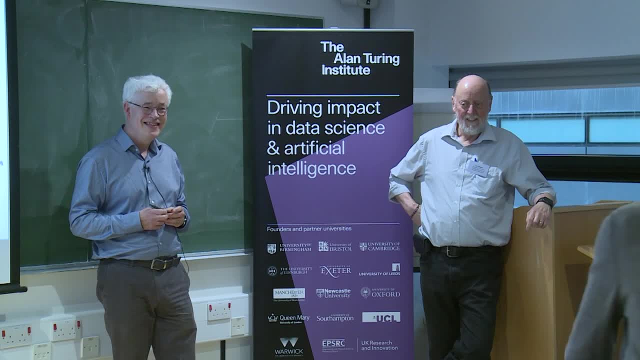 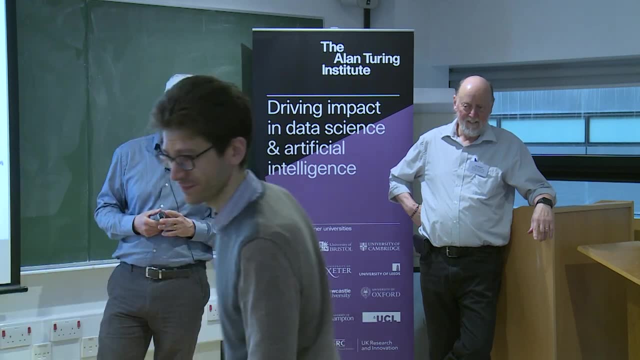 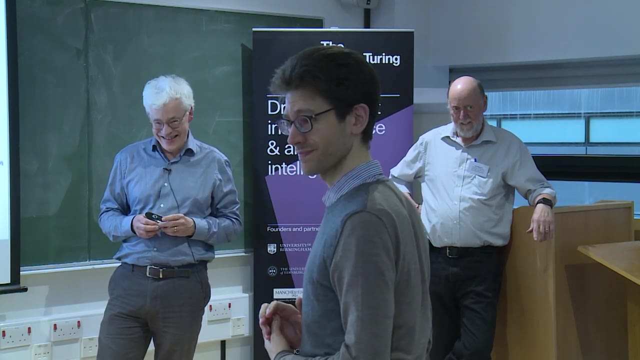 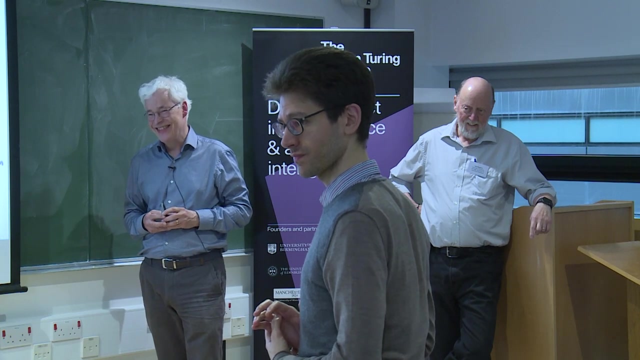 and nobody likes the warners. You look at the internet and computing with floating pointers- mysterious and scary- and you should only use integers and You should never check for equality among floating point numbers. Yeah, That's probably believed around. math works as well. 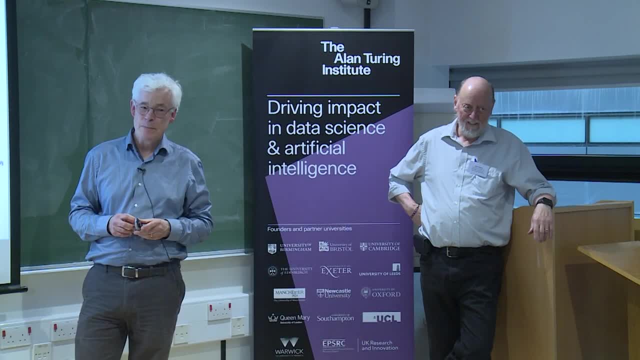 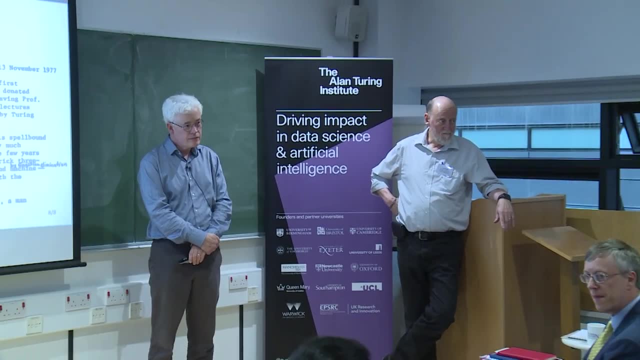 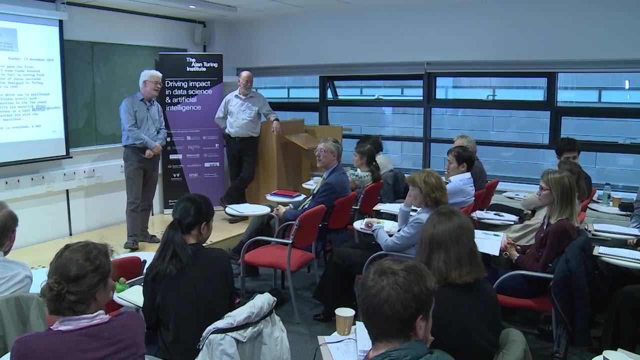 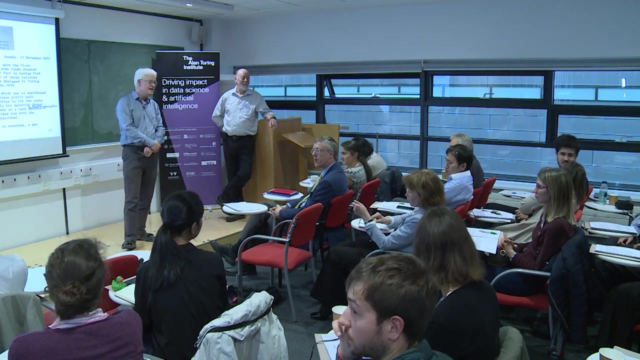 I believe. Yeah. Going back to interval arithmetic, in 1968, Parlette got Khan hired from Toronto to Berkeley and Khan was assigned to teach the graduate numerical analysis course. I fortunately had had it already from Parlette, but Parlette suggested 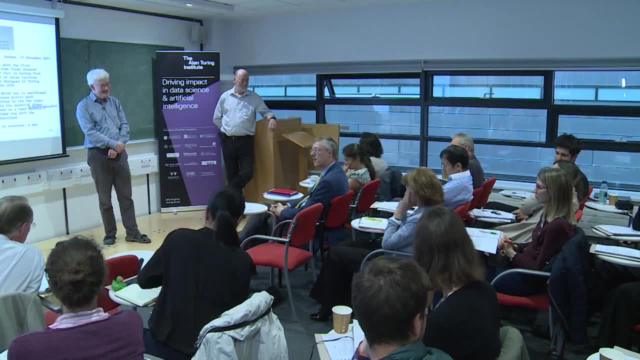 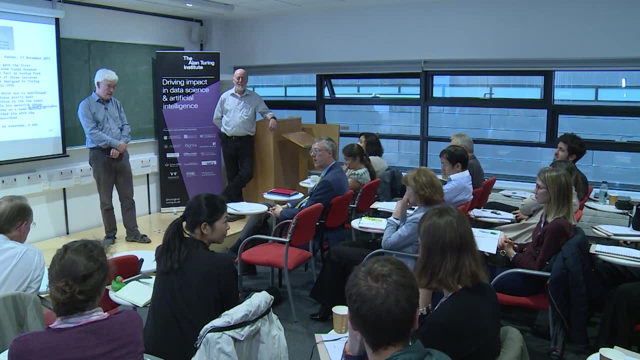 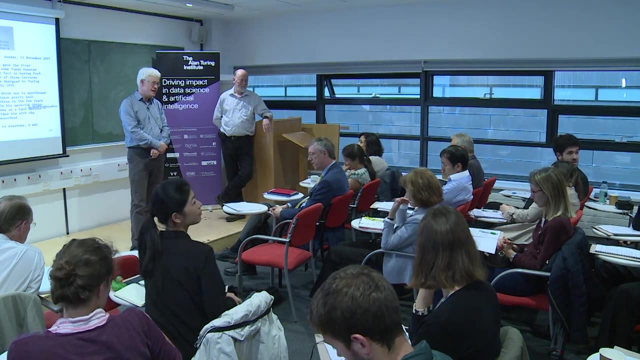 I sit in on Khan's course And Khan taught all of numerical analysis that year using interval arithmetic, Whoa. They were brilliant lectures and terrific work, although my conclusion was that it wasn't really of much use. Was he in a posteriori?